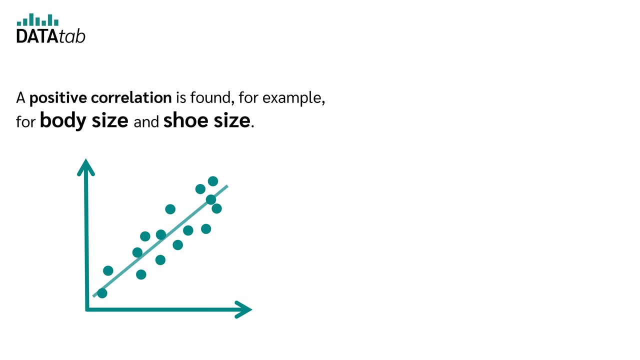 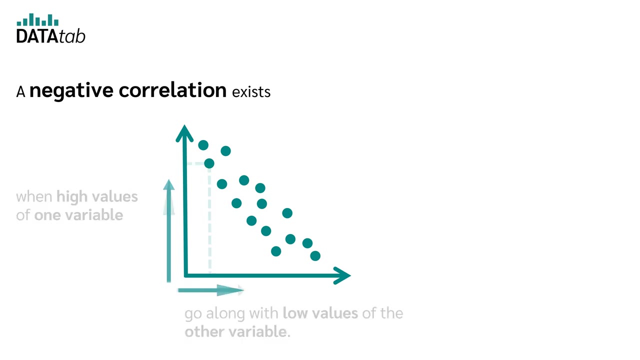 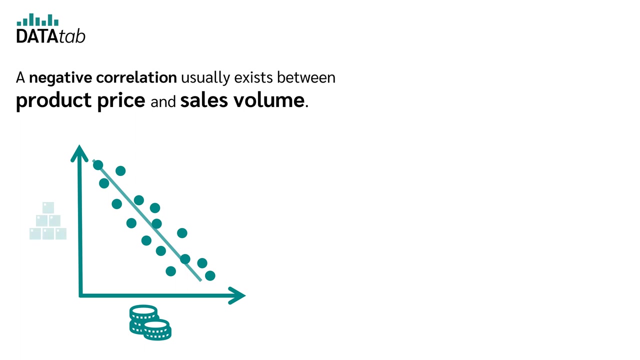 A positive correlation is found, for example, for body size and shoe size. The result is a positive correlation coefficient. A negative correlation exists when high values of one variable go along with low values of the other variable, And vice versa. A negative correlation usually exists between product price and sales volume. 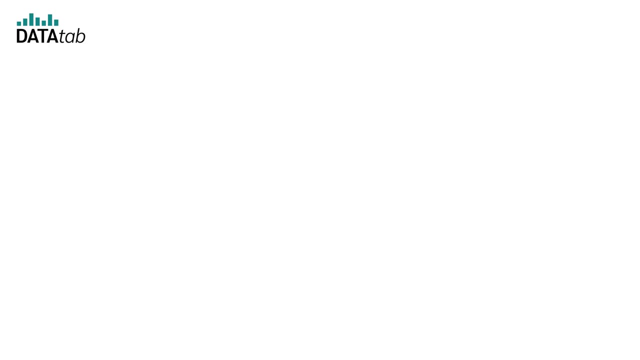 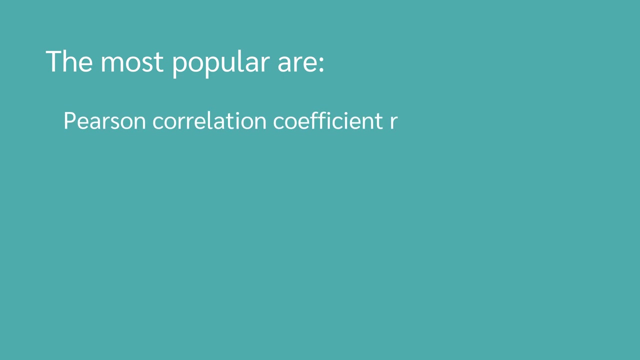 The result is a negative correlation coefficient. Now we have different correlation coefficients. The most popular are Pearson correlation coefficient r, Spearman correlation coefficient rs, Canals, tau and point-by-zero correlation coefficient r. Let's start with the first, the Pearson correlation coefficient. 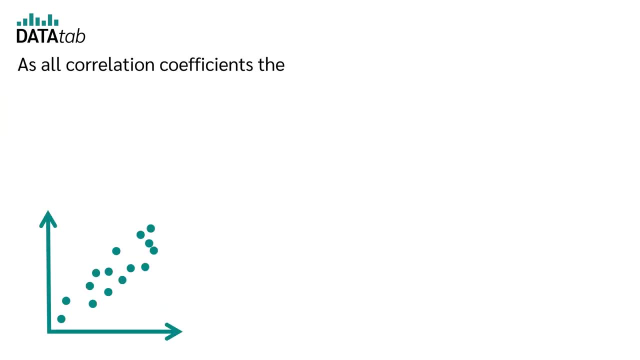 What is a Pearson correlation? As all correlation coefficients, the Pearson correlation r is a statistical measure that quantifies the relationship between two variables. In the case of Pearson correlation, the linear relationship of metric variables is measured. More about metric variables later. So with the help of Pearson correlation, 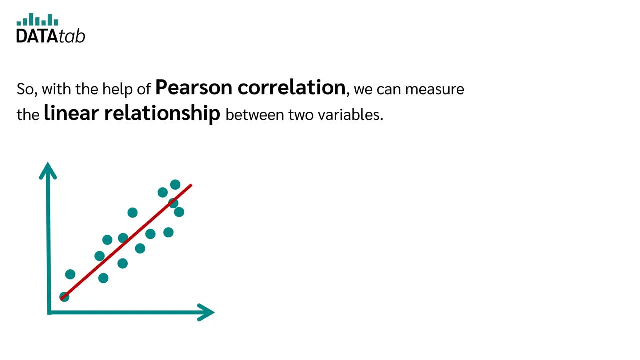 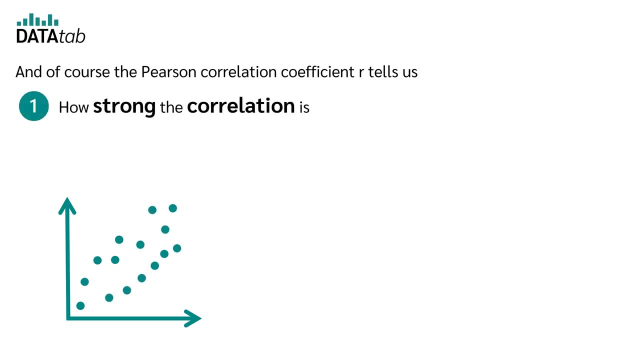 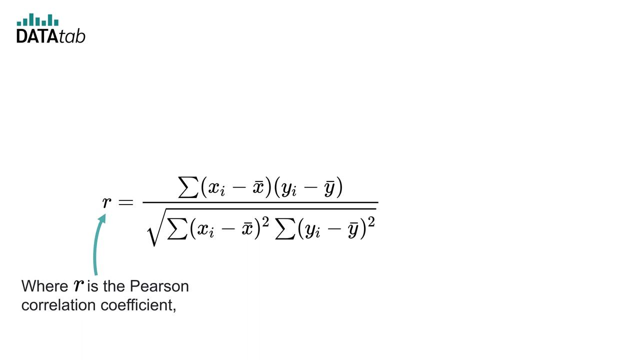 we can measure the linear relationship between two variables And, of course, the Pearson correlation coefficient r tells us how strong the correlation is and in which direction the correlation goes. How is Pearson correlation calculated? The Pearson correlation coefficient is obtained via this equation, Where r is the Pearson correlation coefficient, x, i are the individual values of one variable. 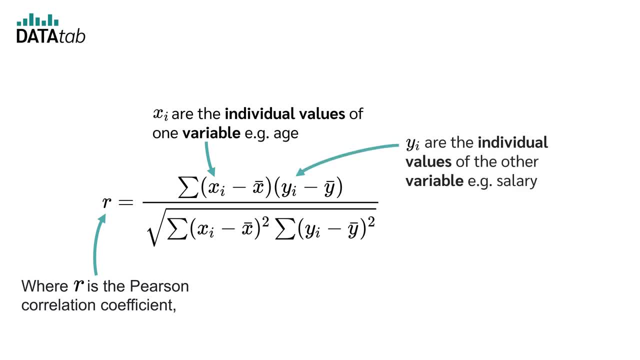 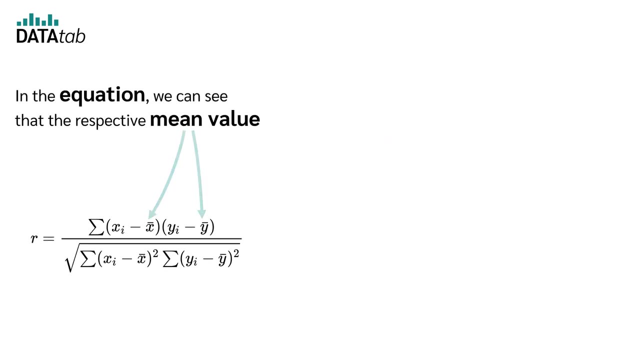 one variable, for example age yi, are the individual values of the other variable, for example salary. x' and y' are respectively the mean values of the two variables. In the equation we can see that the respective mean value is first subtracted from both values. 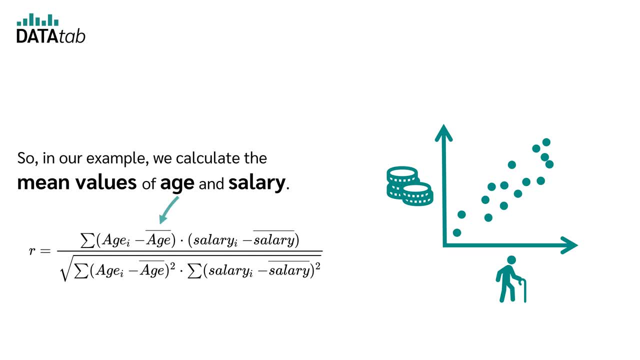 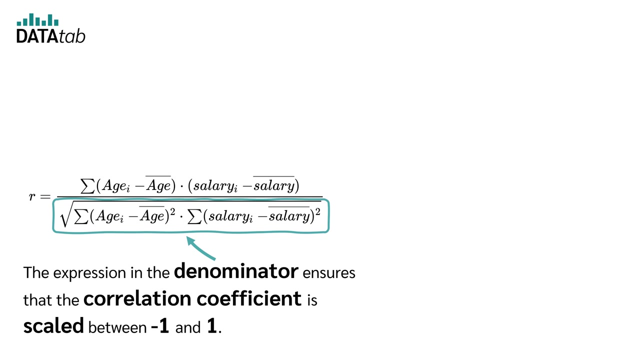 So in our example we calculate the mean values of age and salary. We then subtract the mean values from each person's age and salary, Then we multiply both values and we sum up the individual results of the multiplication. The expression in the denominator ensures that the correlation coefficient is scaled. 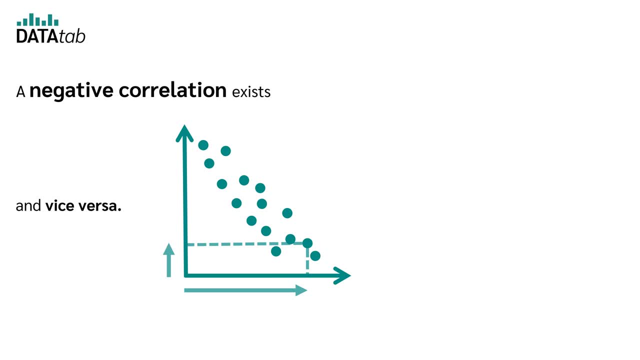 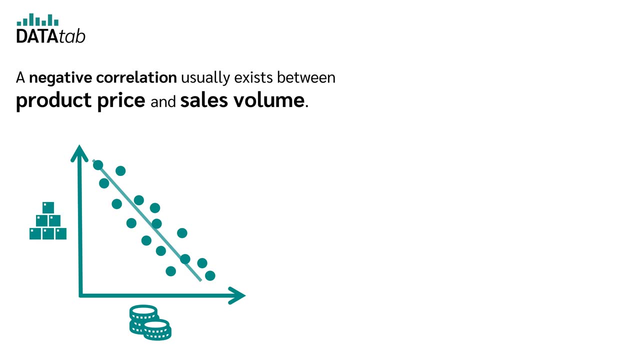 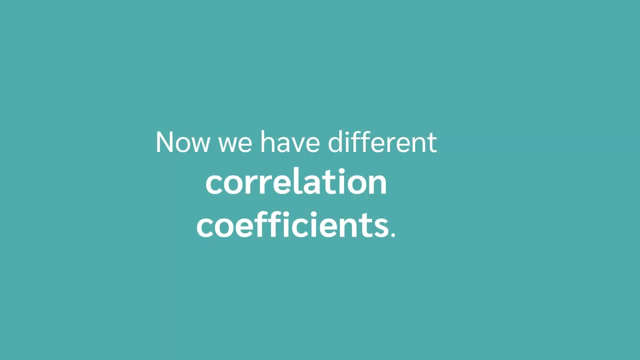 with low values of the other variable and vice versa. A negative correlation usually exists between product price and sales volume. The result is a negative correlation coefficient. Now we have different correlation coefficients. The most popular are Pearson correlation coefficient r, Spearman correlation coefficient rs, Canals, tau and point by zero correlation. 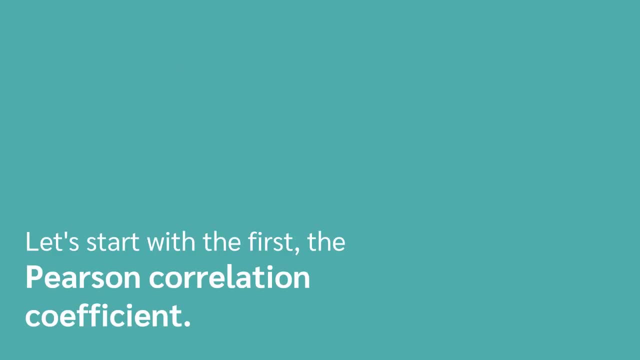 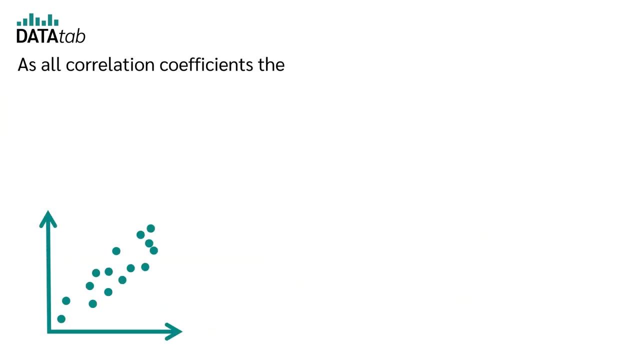 coefficient: rpb. Let's start with the first, the Pearson correlation coefficient. What is a Pearson correlation? As all correlation coefficients, the Pearson correlation r is a statistical measure that quantifies the relationship between two variables. In the case of Pearson correlation, the linear relationship of metric variables is measured. 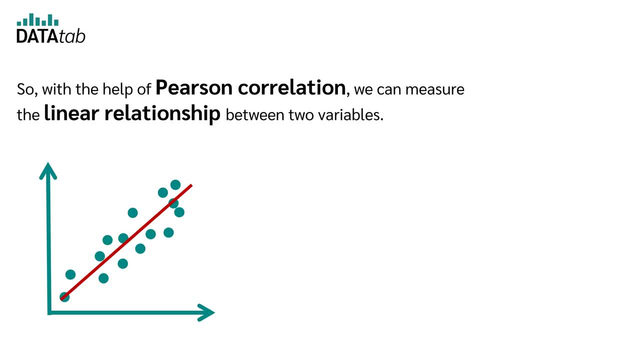 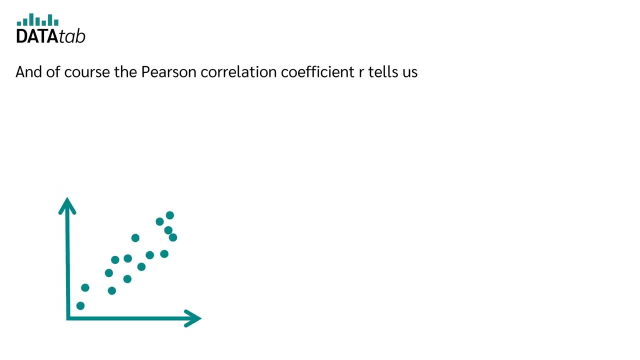 More about metric variables later. So with the help of Pearson correlation we can measure the linear relationship between two variables And of course, the Pearson correlation coefficient r tells us how strong the correlation is and in which direction the correlation goes. How is Pearson? 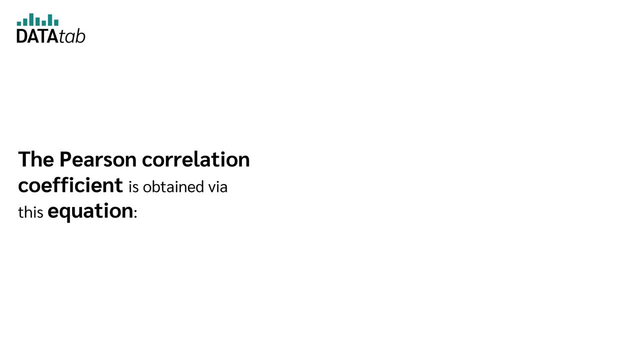 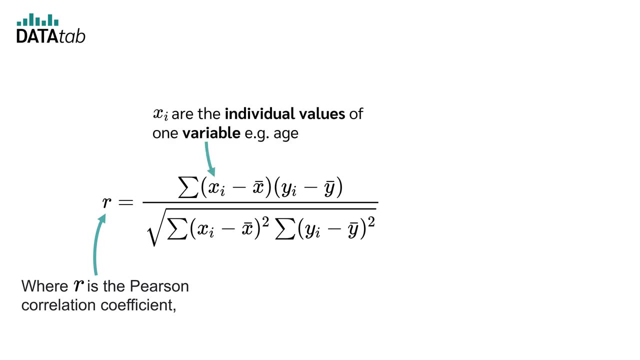 correlation calculated. The Pearson correlation coefficient is obtained via this equation: where r is the Pearson correlation coefficient. xi are the individual values of one variable, for example h. yi are the individual values of the other variable, for example salary. x' and y' are respectively the: 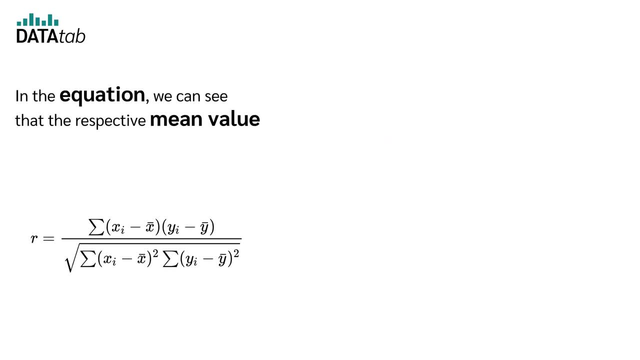 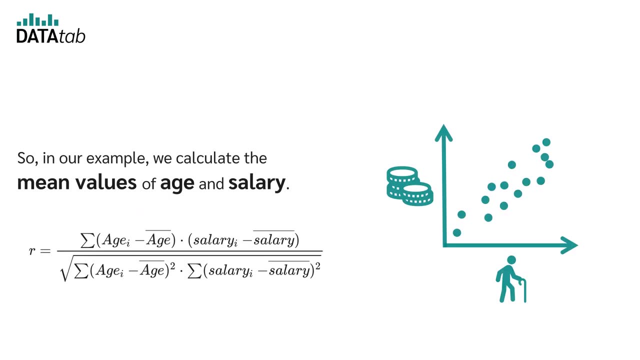 mean values of the two variables. In the equation we can see that the respective mean value is first subtracted from both values. So in our example we calculate the mean values of h and xi. We then subtract the mean values from each person's age and salary. 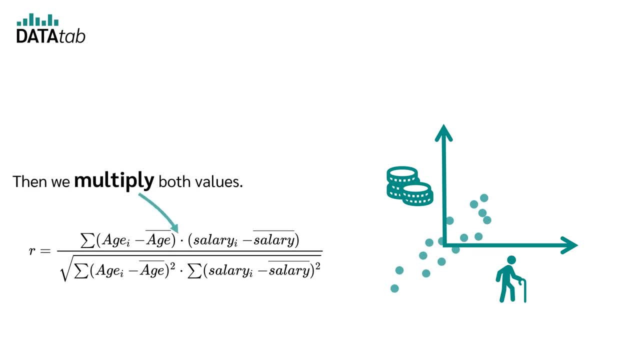 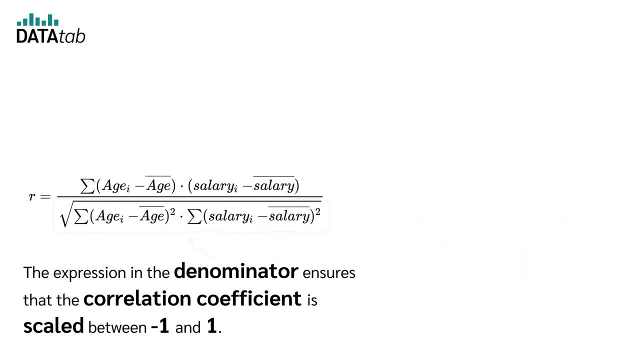 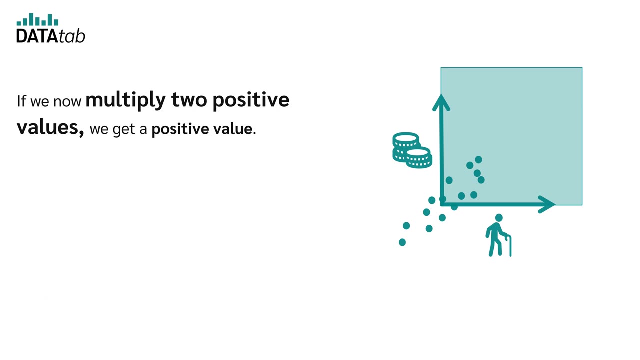 We then subtract the mean values from each person's age and salary, Then we multiply both values and we sum up the individual results of the multiplication. The expression in the denominator ensures that the correlation coefficient is scaled between minus 1 and 1.. If we now multiply two positive 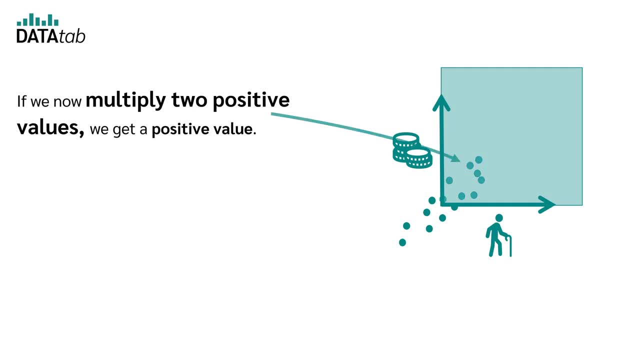 between minus one and one. If we now multiply two positive values, we get a positive value. So all values that lie in this area have a positive influence on the correlation coefficient. If we multiply two negative values, we also get a positive value. 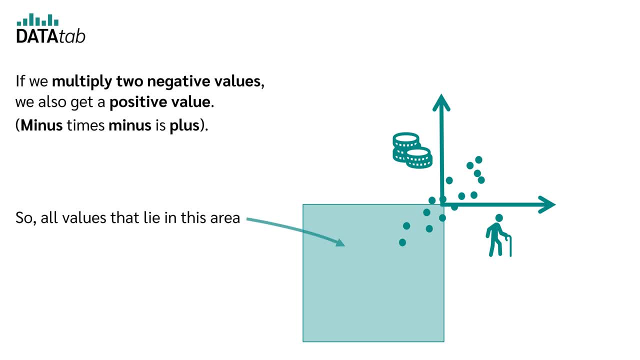 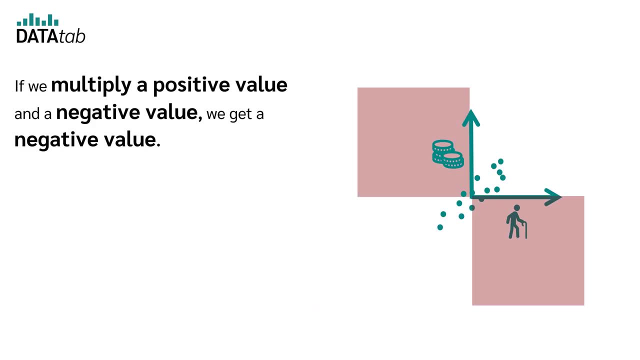 Minus times minus is plus, So all values that lie in this area also have a positive influence on the correlation coefficient. If we multiply a positive value and a negative value, we get a negative value. Minus times minus is minus, So all values that lie in these ranges have a negative influence on the correlation coefficient. 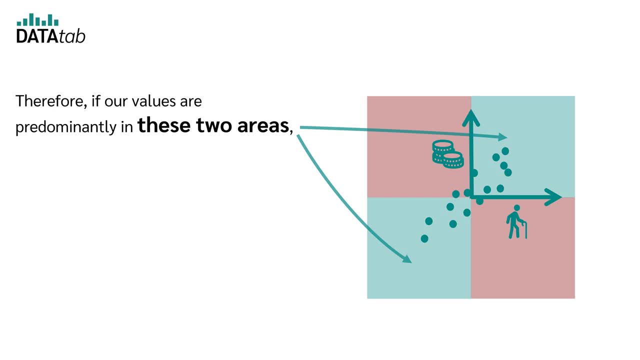 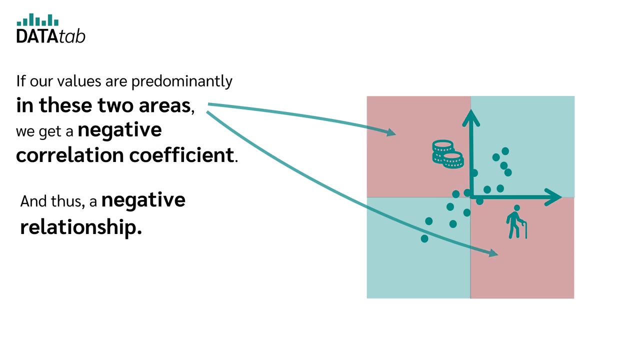 Therefore, if our values are predominantly in these two areas, we get a positive correlation coefficient and thus a positive relationship. If our values are predominantly in these two areas, we get a negative correlation coefficient and thus a negative relationship. If the points are distributed over all four areas- the positive terms and the negative- 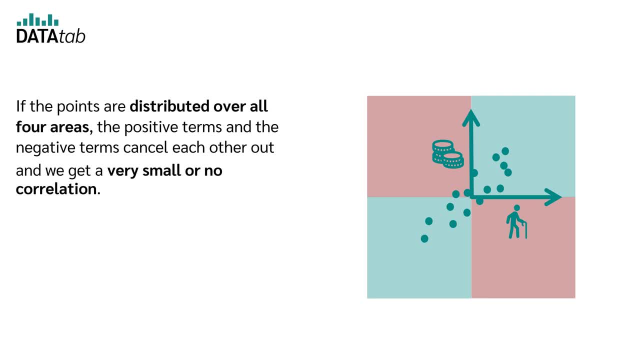 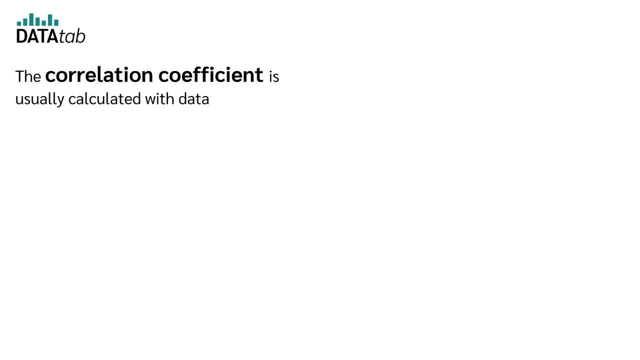 terms cancel each other out and we get a very small or no correlation. But now there's one more thing to consider. The correlation coefficient is usually calculated with data taken from a sample. However, we often want to test a hypothesis about the population. 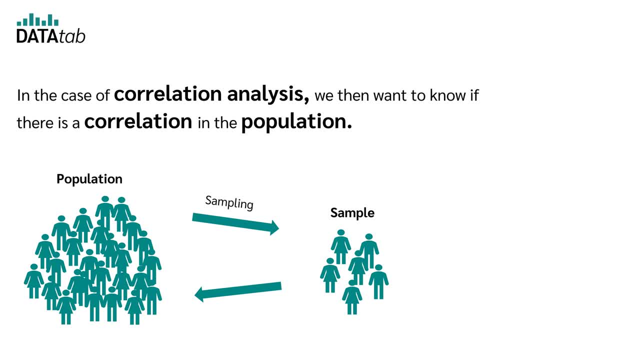 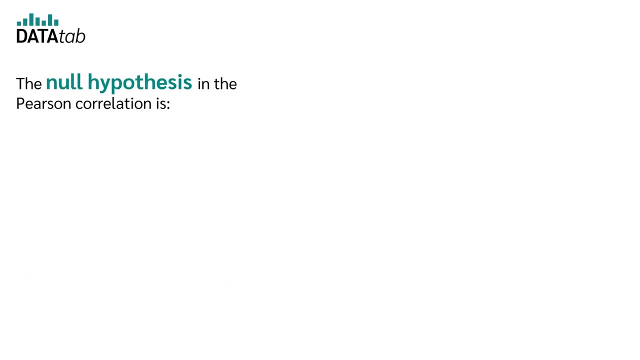 In the case of correlation analysis, we can calculate the correlation coefficient by the formula E. We then want to know if there is a correlation in the population. For this we check whether the correlation coefficient in the sample is statistically significantly different from zero. 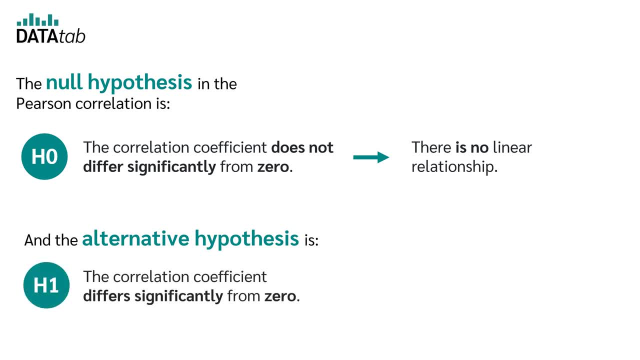 The null hypothesis in the Pearson correlation is: The correlation coefficient does not differ significantly from zero. There is no linear relationship from zero. There is a linear relationship. Attention: It is always tested whether the null hypothesis is rejected or not. In our example, the research question is: 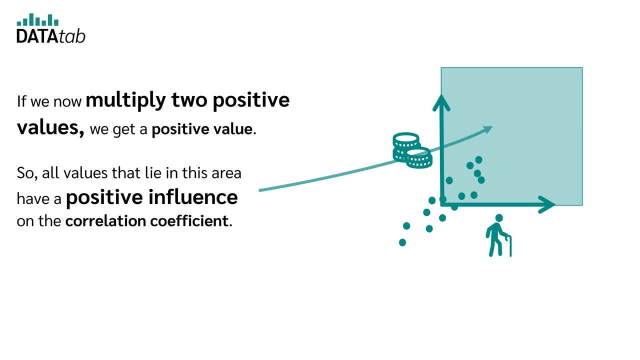 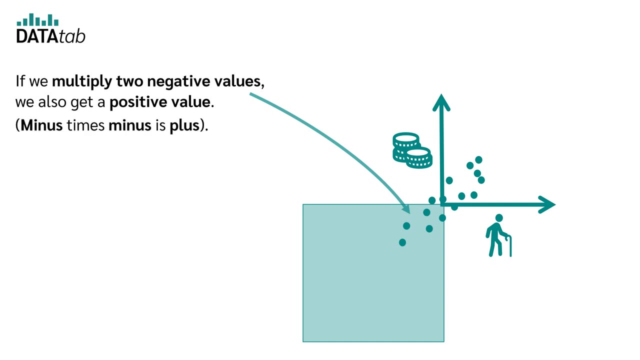 values, we get a positive value, So all values that lie in this area have a positive influence on the correlation coefficient. If we multiply two negative values, we also get a positive value. Minus times minus is plus, So all values that lie in this area also have a positive influence on the correlation coefficient. 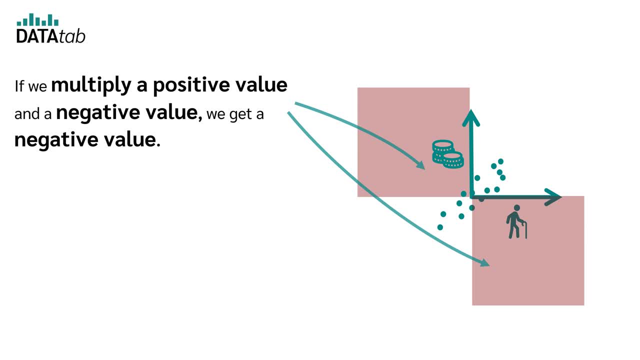 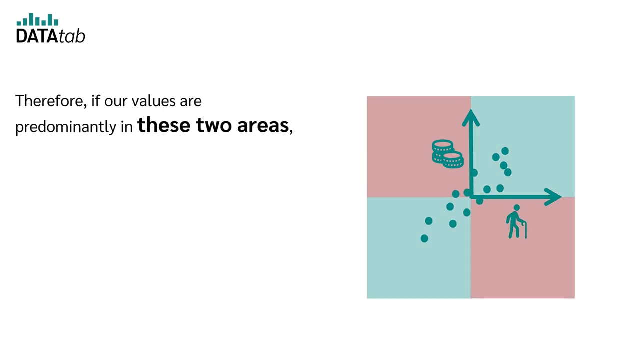 If we multiply a positive value and a negative value, we get a negative value. Minus times plus is minus, So all values that lie in these ranges have a negative influence on the correlation coefficient. Therefore, if our values are predominantly in these two areas, we get a. 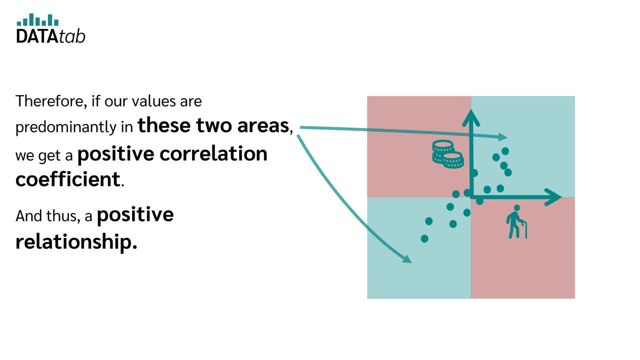 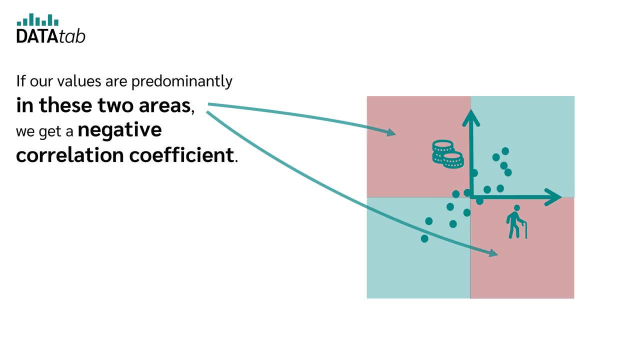 positive correlation coefficient and thus a positive relationship. If our values are predominantly in these two areas, we get a negative correlation coefficient and thus a negative relationship. If the points are distributed over all four areas, the positive terms and the negative terms cancel each other out and 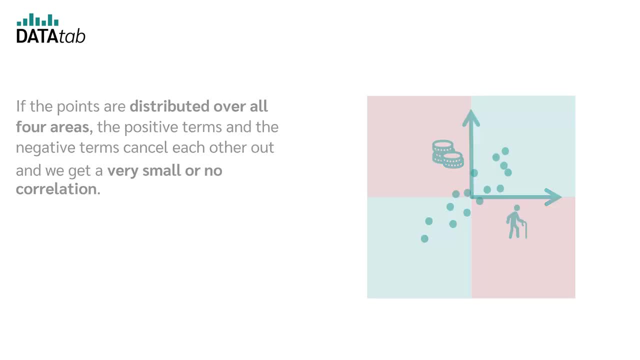 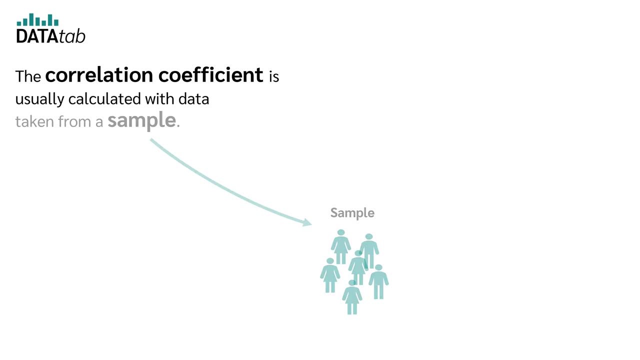 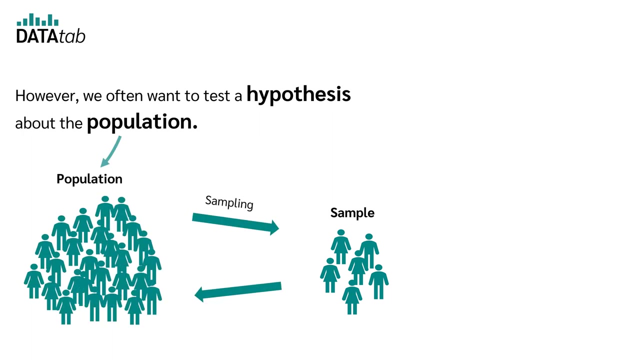 we get a very small or no correlation. But now there's one more thing to consider. The correlation coefficient is usually calculated with data taken from a sample. However, we often want to test a hypothesis about a population. In the case of correlation analysis, we then want to know if there is a correlation. 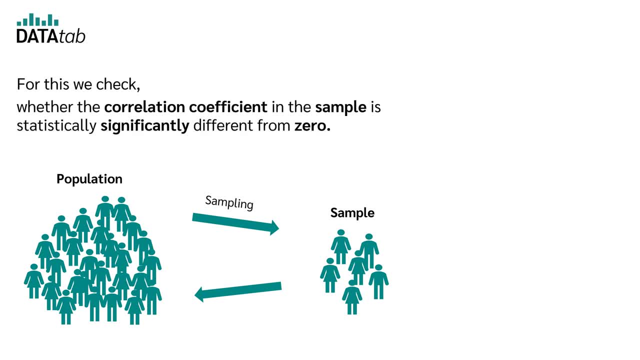 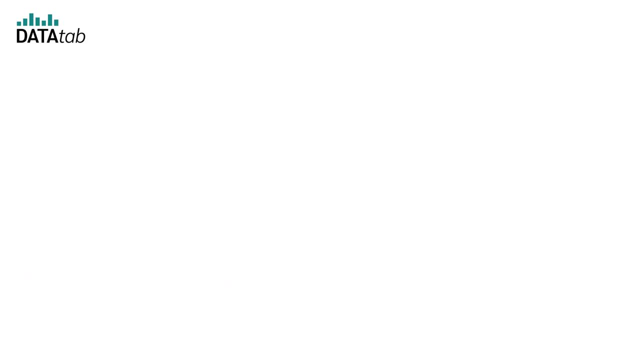 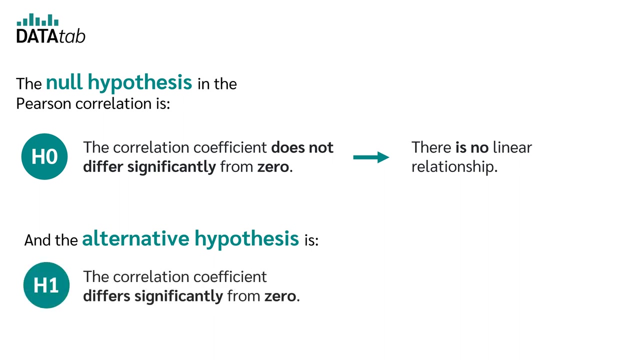 in the population. For this we check whether the correlation coefficient in the sample is statistically significantly different from zero. The null hypothesis in the Pearson correlation is the correlation coefficient does not differ significantly from the correlation coefficient. There is no linear relationship And the alternative hypothesis is the correlation. 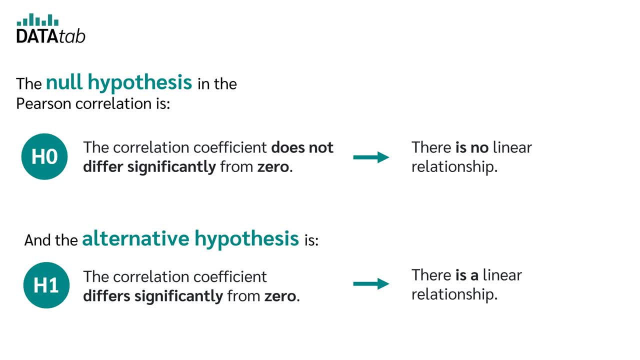 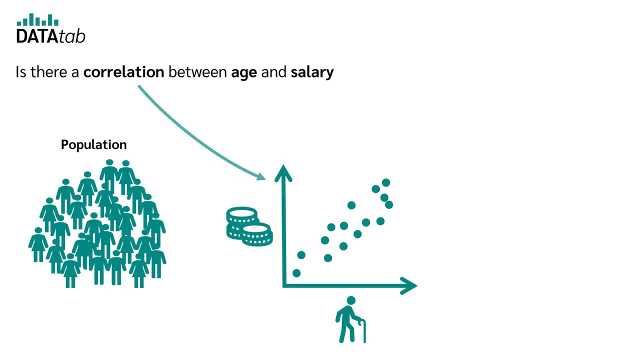 coefficient differs significantly from zero. There is a linear relationship. Attention, It is always tested whether the null hypothesis is rejected or not. In our example, the research question is: is there a correlation between age and salary in the British population? To find out, we draw a line. 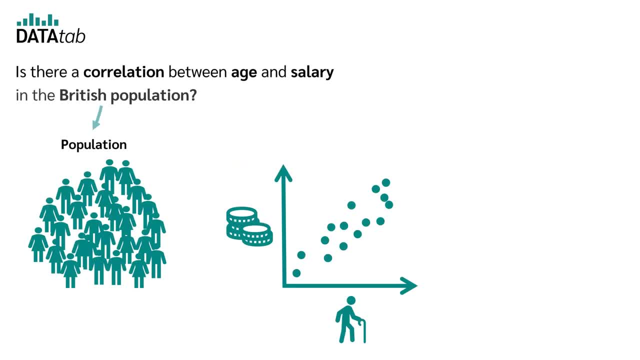 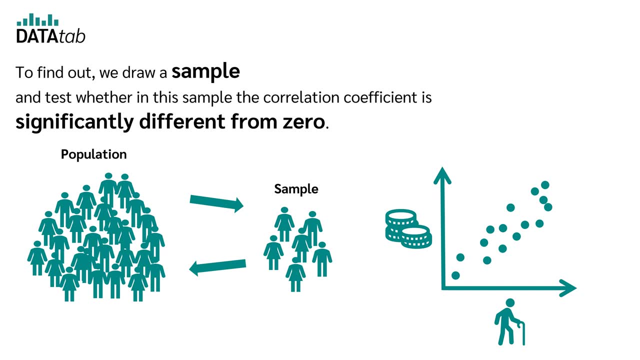 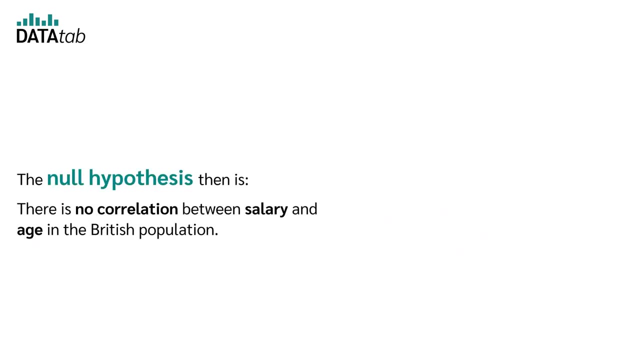 is there a correlation between age and salary in the British population? To find out, we draw a sample and test whether, in this sample, the correlation coefficient is significantly different from zero. The null hypothesis then is there is no correlation between salary and age in the British population. And the alternative hypothesis: there is a correlation between salary. 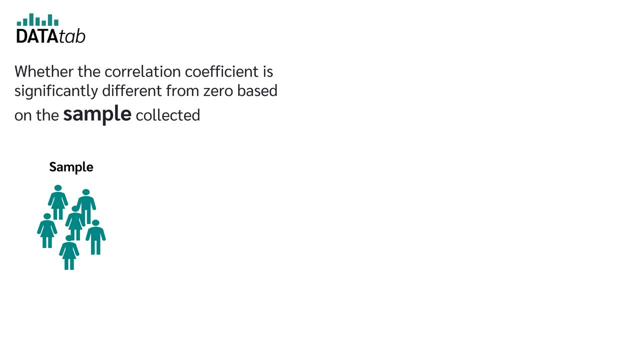 and age in the British population. Whether the correlation coefficient is significantly different from zero based on the sample collected can be checked using a t-test where r is the correlation coefficient and n is the sample size. A p-value can then be calculated from the test statistic t. 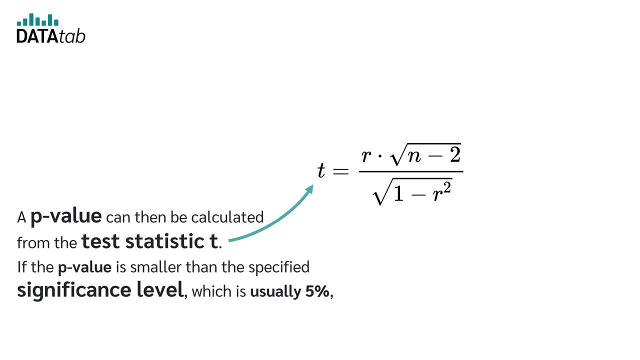 If the p-value is smaller than the specified significance level, which is usually 5%, then the null hypothesis is rejected. Otherwise it is not. But what about the assumptions for a Pearson correlation? Here we must distinguish whether we just want to calculate the Pearson correlation or whether we want to test a hypothesis. 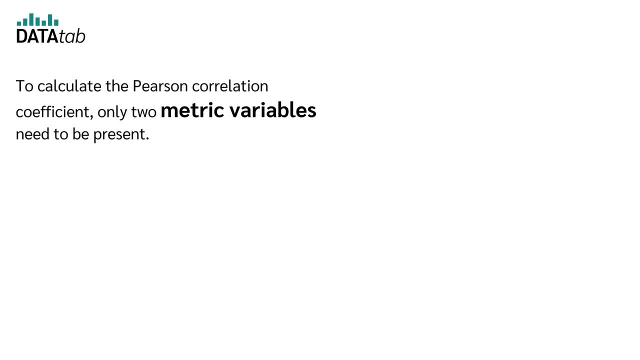 To calculate the Pearson correlation coefficient, only two metric variables need to be present. Metric variables are, for example, a person's weight, a person's salary or electricity consumption. The Pearson correlation coefficient then tells us how large the linear relationship is. 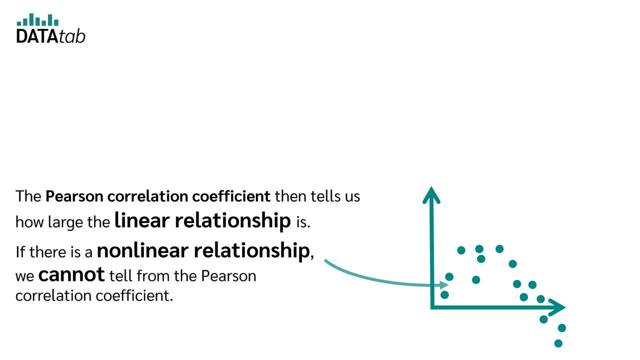 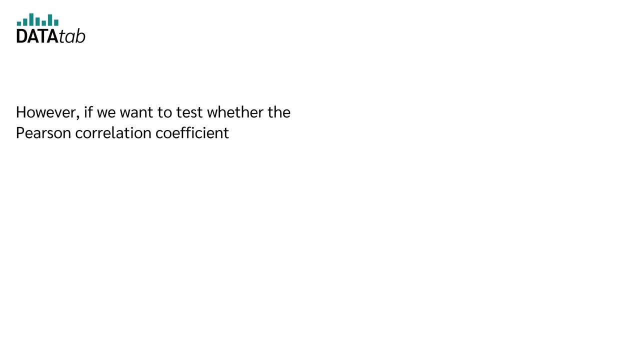 If there is a non-linear relationship, we cannot tell from the Pearson correlation coefficient. However, if we want to test whether the Pearson correlation coefficient is larger than the Pearson correlation coefficient is significantly different from zero, the two variables must always be normally distributed. If this is not given, the calculated test statistic. 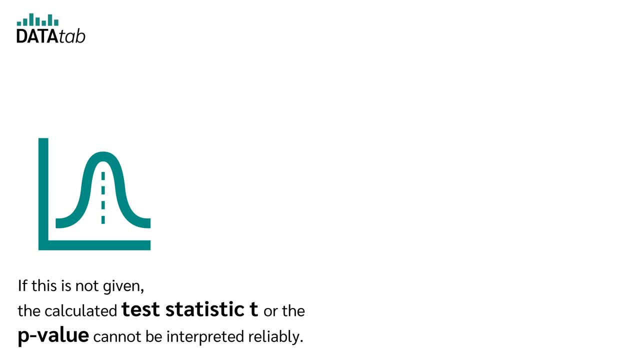 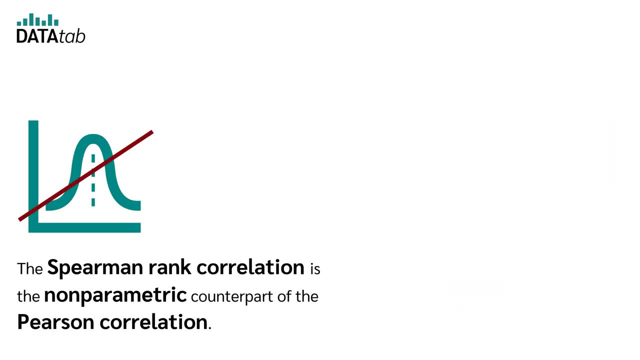 t or the p-value cannot be interpreted reliably. Let's continue with the Spearman correlation. The Spearman-Rang correlation is the non-parametric counterpart of the Pearson correlation, But there is an important difference between the Pearson correlation coefficient and the Pearson correlation coefficient. 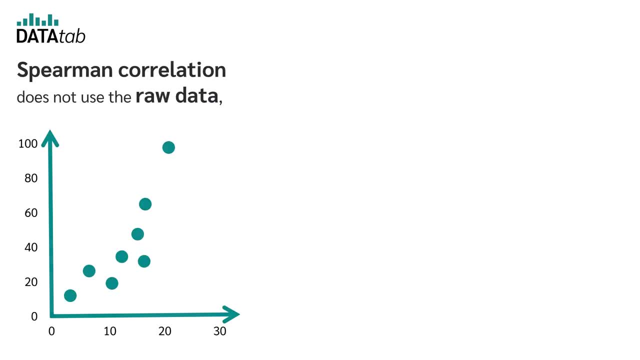 Spearman correlation does not use the raw data, but the ranks of the data. Spearman correlation does not use raw data, but the ranks of the data. Let's look at this with an example. We measure the reaction time of 8 computer players and. 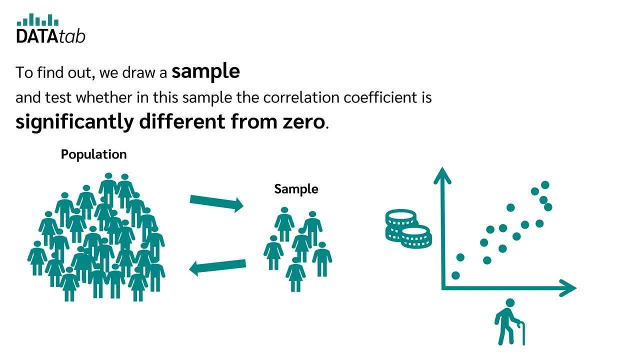 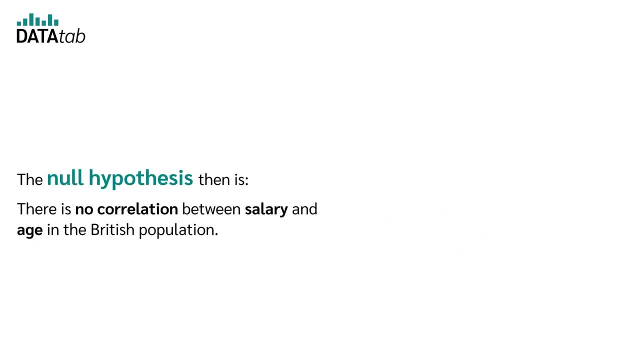 We draw a sample and test whether, in this sample, the correlation coefficient is significantly different from zero. The null hypothesis then is there is no correlation between salary and age in the British population. And the alternative hypothesis: there is a correlation between salary and age in. 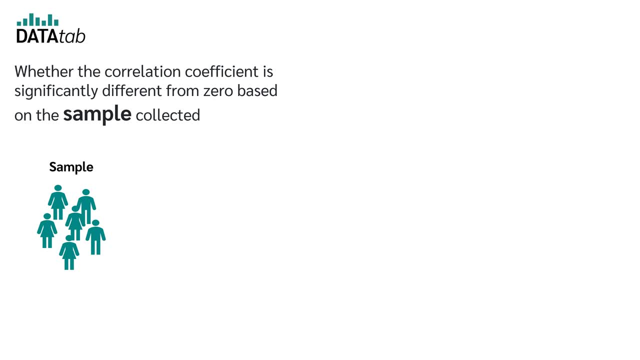 the British population. Whether the correlation coefficient is significantly different from zero based on the sample collected can be checked using a t-test, where r is the correlation coefficient and n is the sample size. A p-value can then be calculated from the test statistic t. If the p-value is 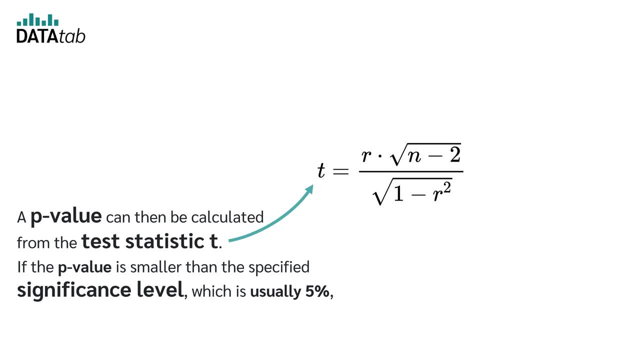 smaller than the specified significance level, which is usually 5%, then the null hypothesis is rejected, otherwise it is not. But what about the assumptions for a Pearson correlation? Here we must distinguish whether we just want to calculate the Pearson correlation or whether we want to test a hypothesis. 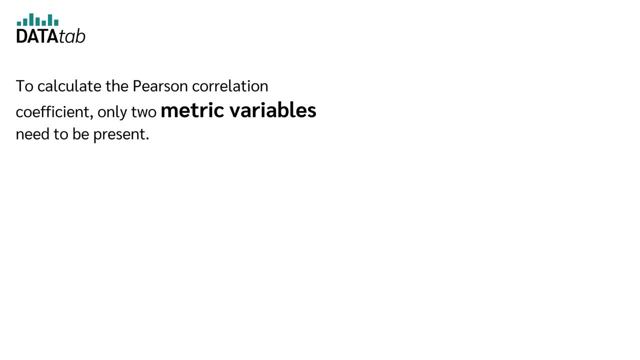 To calculate the Pearson correlation coefficient, only two metric variables need to be present. Metric variables are, for example, a person's weight, a person's salary or electricity consumption. The Pearson correlation coefficient then tells us how large the linear relationship is If there is a non-linear relationship. 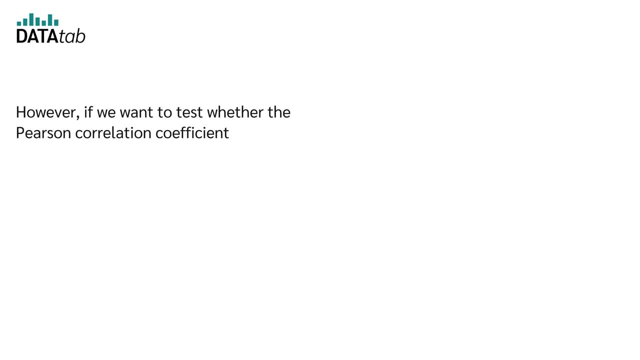 we cannot tell from the Pearson correlation coefficient. However, if we want to test whether the Pearson correlation coefficient is significantly different from zero, the two variables must always be normally distributed. If this is not given, the calculated test statistic t or the p-value cannot be interpreted reliably. Let's continue with the Spearman correlation. 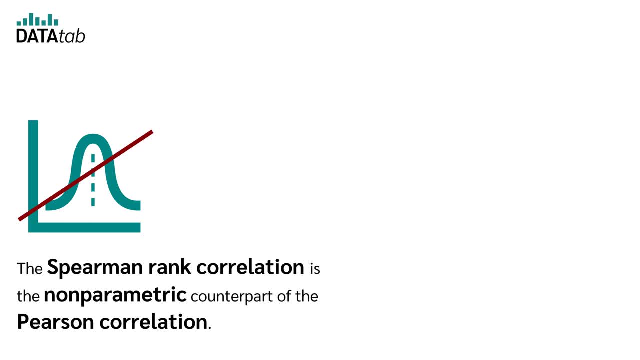 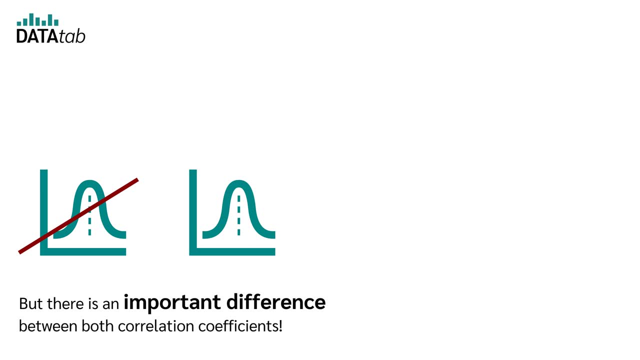 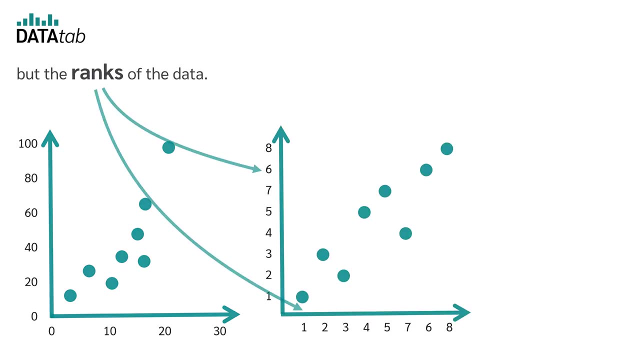 The Spearman-Wrang correlation is, for example, the number of hours a person spends on the computer. This is the non-parametric counterpart of the Pearson correlation, But there is an important difference between both correlation coefficients. Spearman correlation does not use the raw data, but the ranks of the data. Let's look at this with an example. We measure 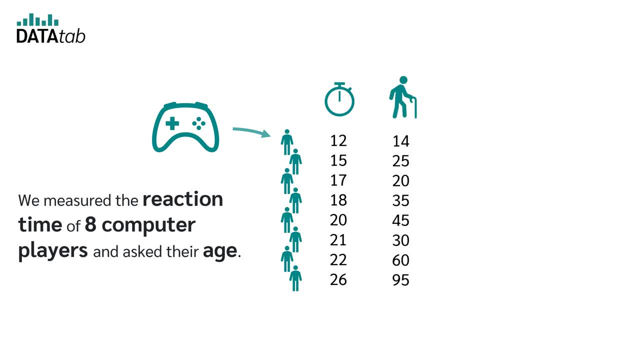 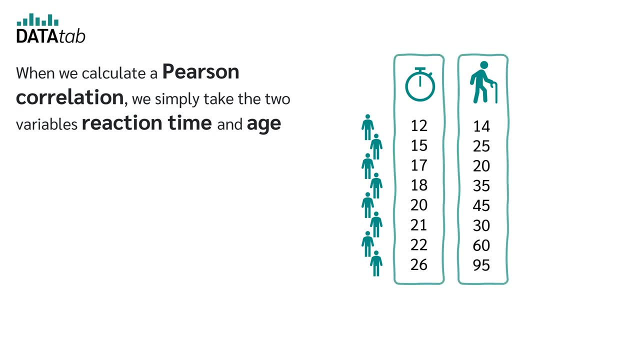 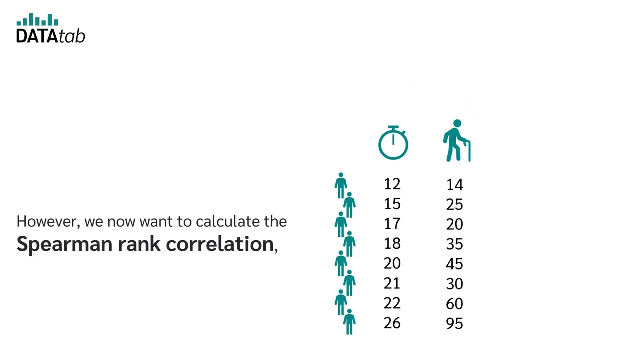 the reaction time of 8 computer players and ask their age. When we calculate a Pearson correlation, we simply take the two variables, reaction time and age, and calculate the Pearson correlation coefficient. However, we now want to calculate the Spearman-Wrang correlation. So first we assign a rank to each person for reaction. 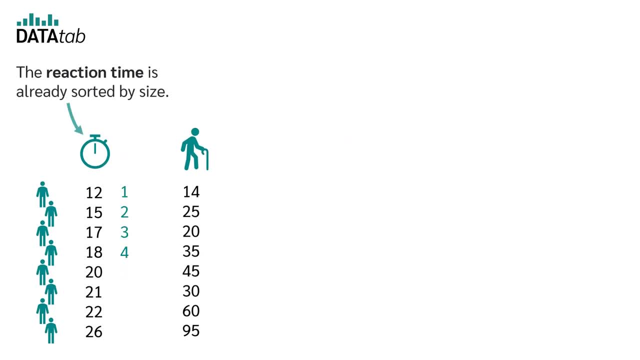 time and age. The reaction time is already sorted by size. 12 is the smallest value, so gets ranked 1.. 15, the second smallest value, so gets ranked rank 2, and so on and so forth. We are now doing the same with age. Here we have the. 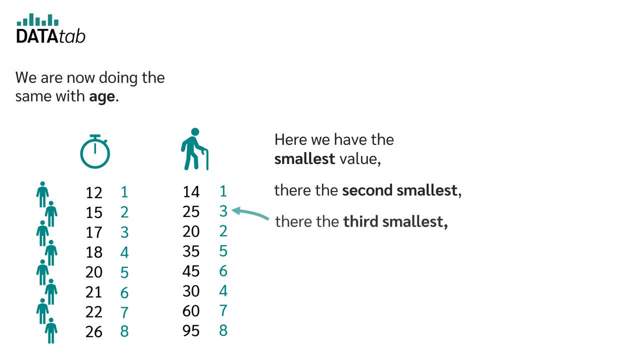 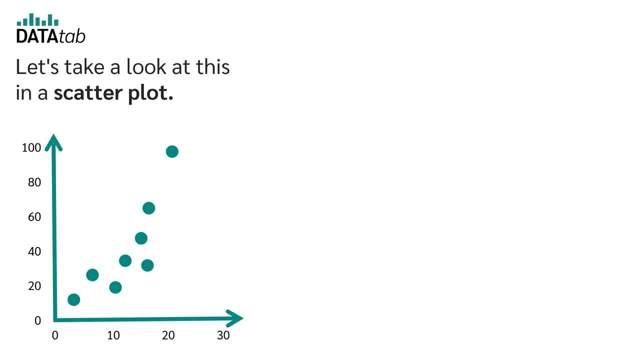 smallest value there, the second smallest there, the third smallest, fourth smallest, and so on and so forth. Let's take a look at this in the scatter plot. Here we see the raw data of age and reaction time. But now we would like to use the. 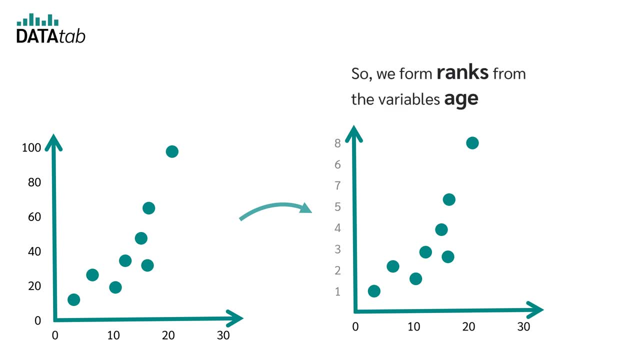 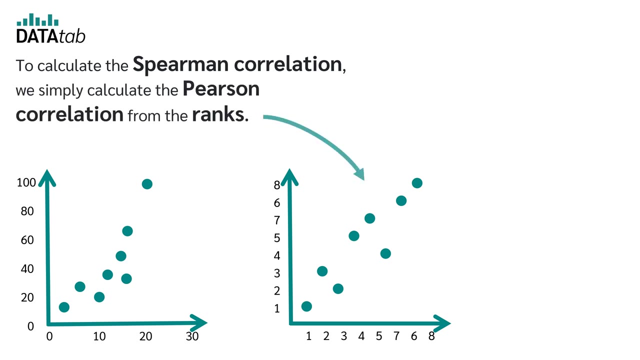 rankings. So we form ranks from the variables age and reaction time. Through this transformation we have now distributed the data more evenly. To calculate the Pearson correlation, we simply calculate the Pearson correlation from the ranks, So the Spearman correlation is equal to the Pearson. 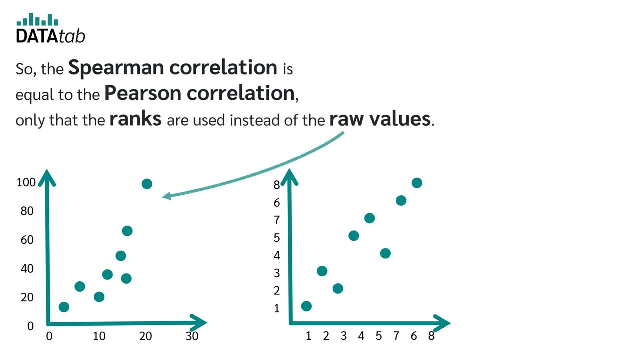 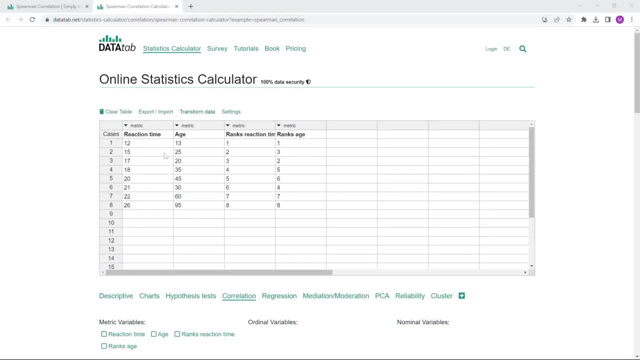 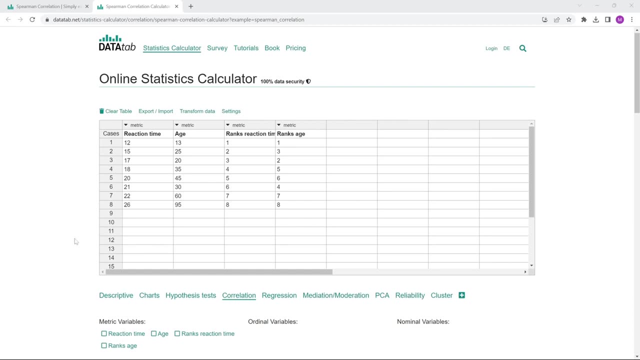 correlation, only that the ranks are used instead of the raw value. Let's have a quick look at that in DataTab. Here we have the reaction time and age and there we have the just created ranks of reaction time and age. Now we can either calculate: 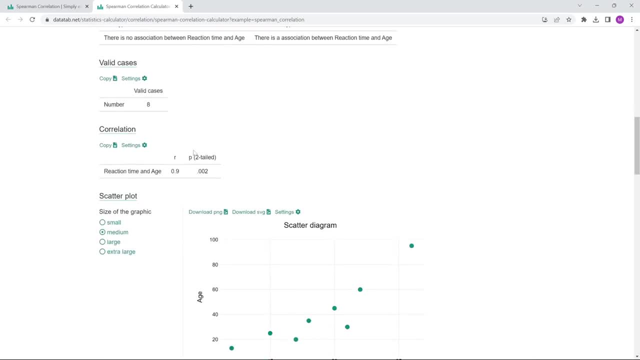 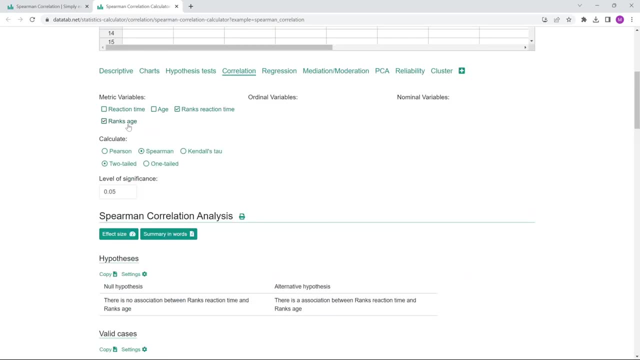 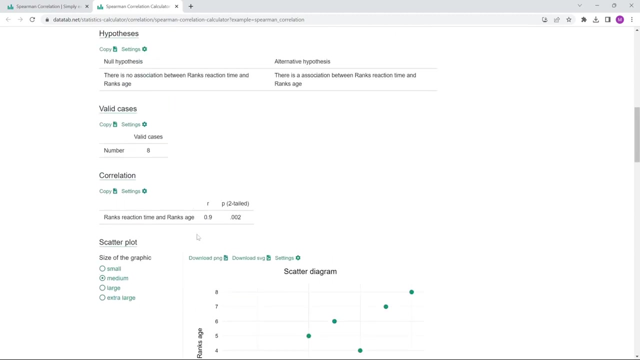 Spearman correlation of reaction time and age, where we get a correlation of 0.9. or we can calculate Pearson correlation from the ranks, where we also get 0.9.. So exactly the same. If you like, you can download the dataset. You can find the link in the video description. 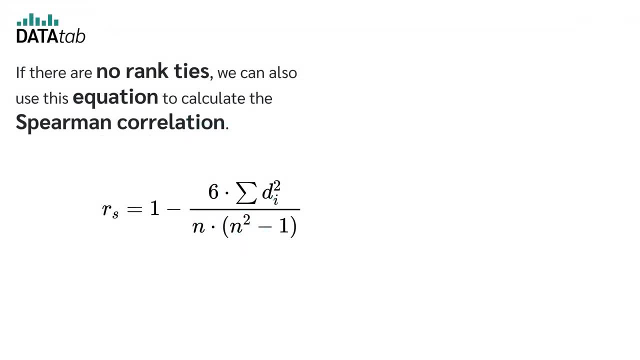 If there are no rank ties, we can also use this equation to calculate the Pearson correlation. RS is the Spearman correlation, N is the number of cases and D is the difference in ranks between the two variables. Referring to our example, we get the different Ds with this: 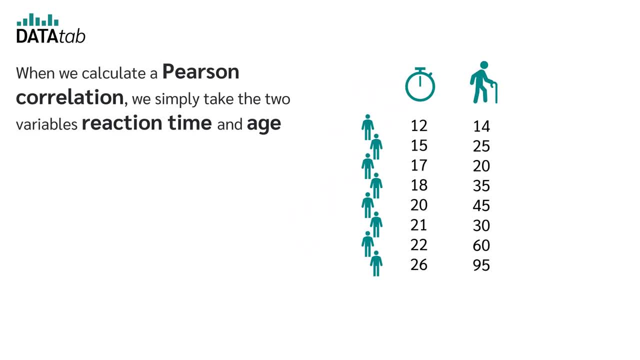 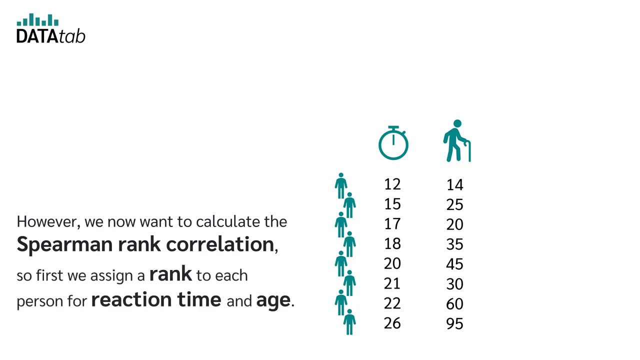 ask their age. When we calculate a Pearson correlation we simply take the two variables reaction time and age and calculate the Pearson correlation coefficient. Spearman correlation is more than just anرation. The Pearson correlation coefficient is more than We now want to calculate the Spearman rank correlation. so first we assign a rank to 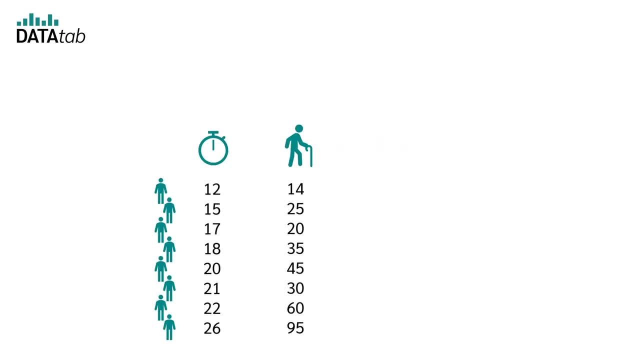 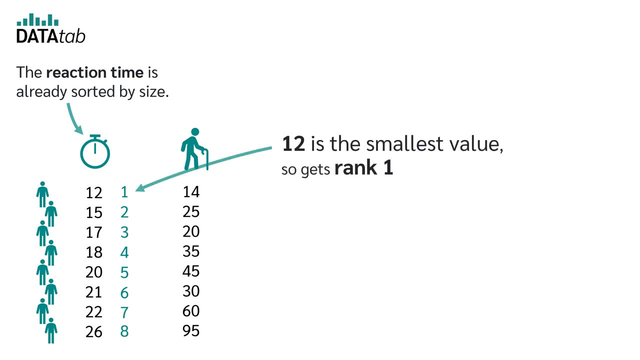 each person for reaction time and age. The reaction time is already sorted by size: 12 is the smallest value, so gets rank 1, 15 the second smallest value, so gets rank 2, and so on and so forth. We are now doing the same with age. 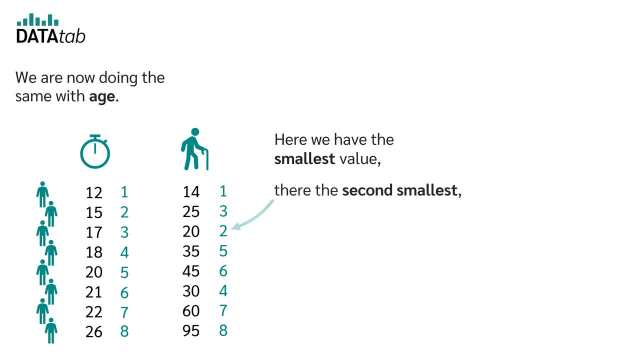 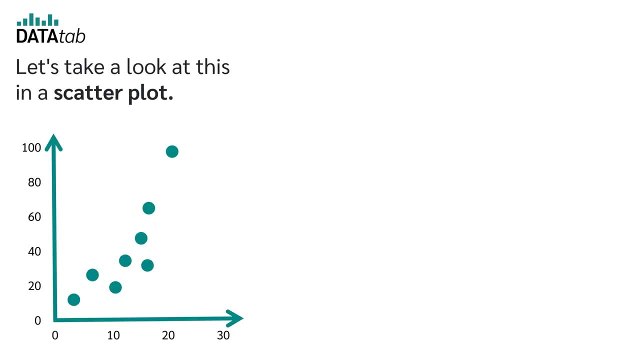 Here we have the smallest value there, the second smallest, there the third smallest, fourth smallest and so on and so forth. Let's take a look at this in the scatterplot. Here we see the raw data of age and reaction time. But now we would like to use the rankings. 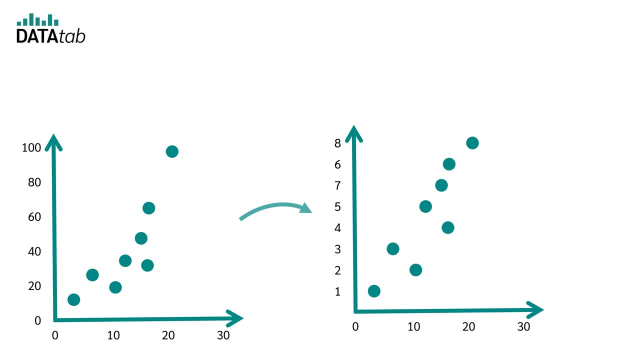 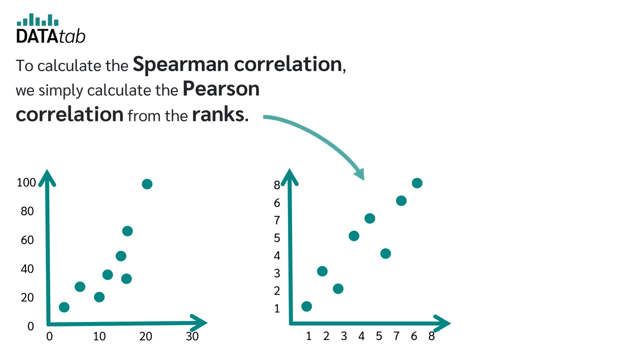 So we form ranks from the variables age and reaction time. Through this transformation we have now distributed the distribution. We can now calculate the data more evenly. To calculate the Pearson correlation, we simply calculate the Pearson correlation from the ranks. So the Spearman correlation is equal to the Pearson correlation, only that the ranks are. 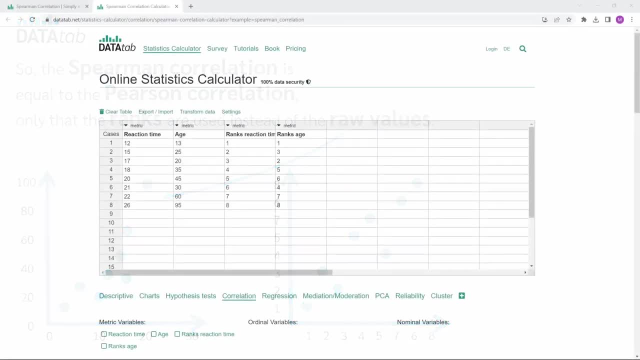 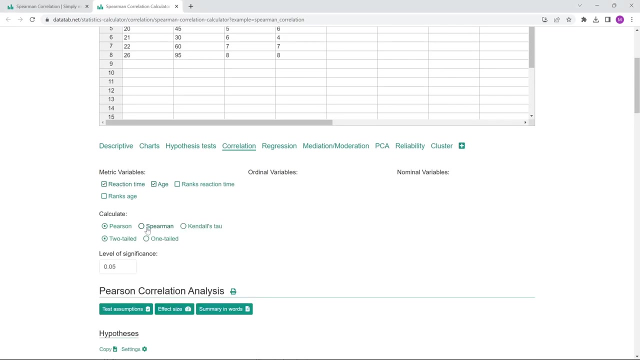 used instead of the raw values. Let's have a quick look at that. in data tab, Here we have the reaction time and age and there we have the just created ranks of reaction time and age. Now we can either calculate Spearman correlation of reaction time and age, where we get a correlation? 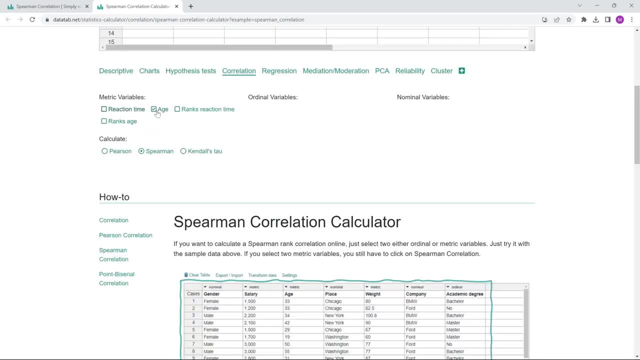 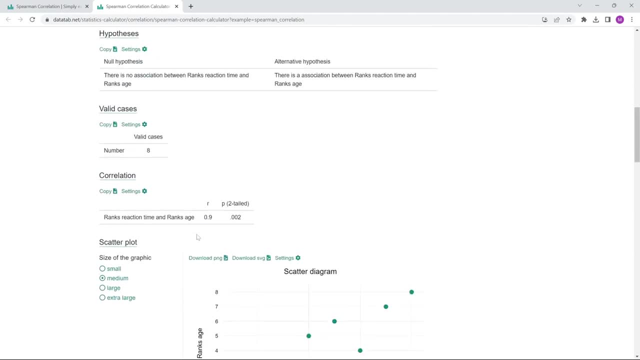 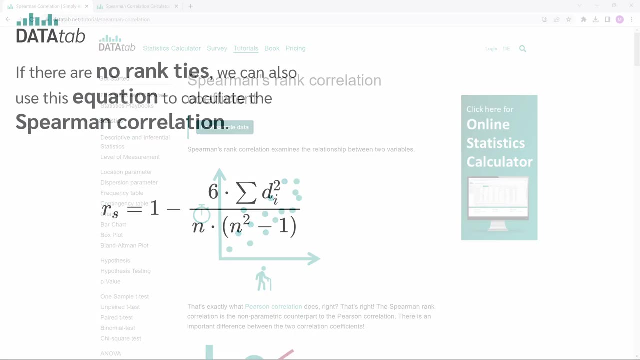 of 0.9.. Or we can calculate Pearson correlation from the ranks, where we also get 0.9.. So exactly the same as before. If you like, you can download the dataset. you can find the link in the video description. 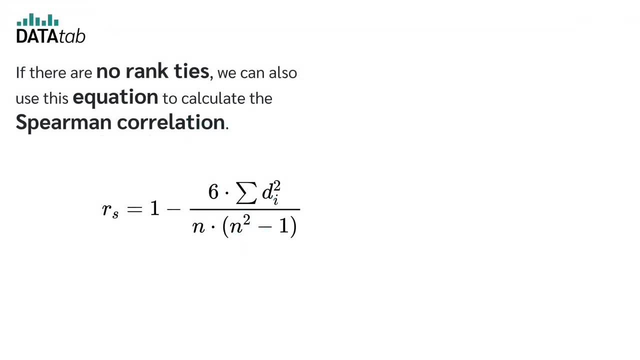 If there are no rank ties, we can also use this equation. Here we have the rank ties. We can also use this equation to calculate the Pearson correlation. Our s is the Spearman correlation: n is the number of cases and d is the difference in. 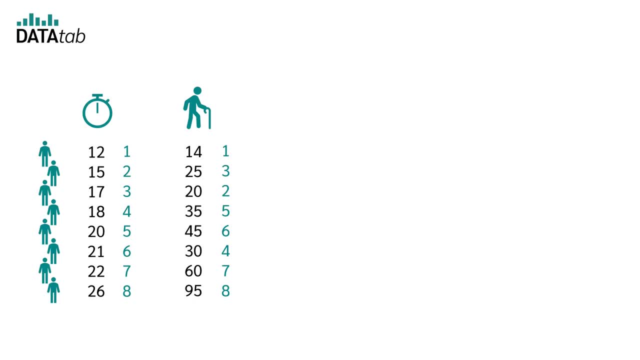 ranks between the two variables. Referring to our example, we get the different d's with this: One minus one is equal to zero, two minus three is minus one, three minus two is one, and so on. Now we square the individual d's and add them all up. 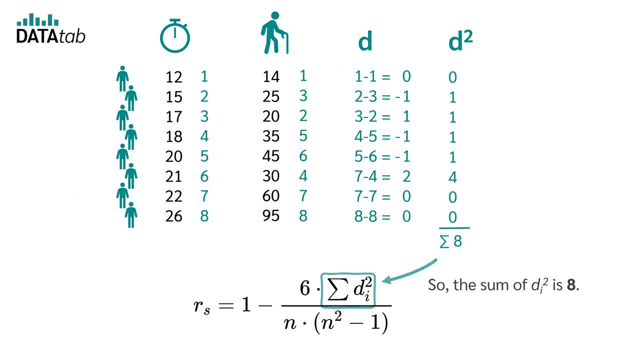 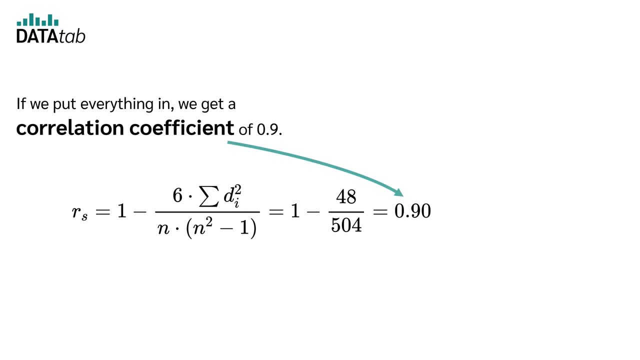 So the sum of d i squared is eight. n, which is the number of people, is eight. If we put everything in, we get a correlation coefficient of 0.9.. Just like the Pearson correlation coefficient r, Spearman correlation coefficient r s also. 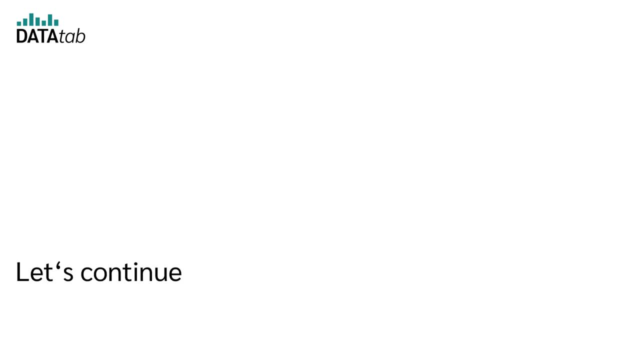 varies between minus one and one. Let's continue with Kendall's tau. Kendall's tau is a correlation coefficient And this does a measure of the correlation coefficient, And this does a measure of the correlation coefficient And this does a measure of the relationship between two variables. 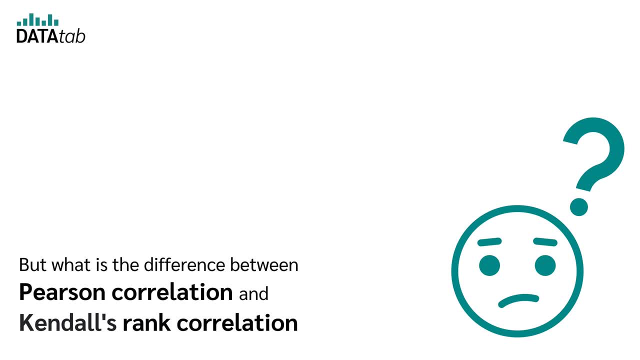 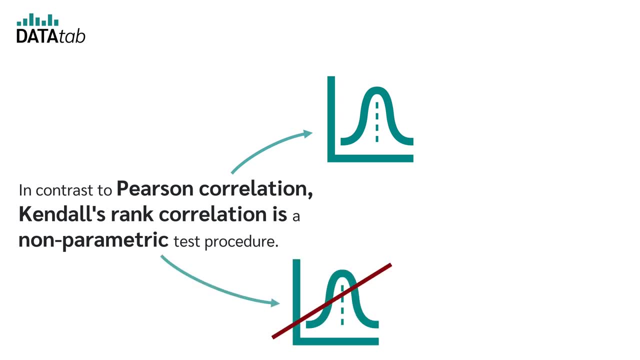 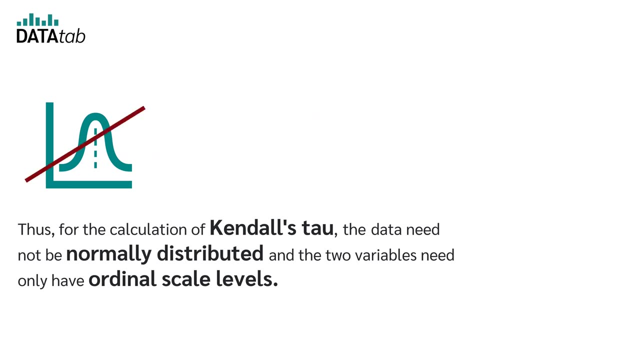 But what is the difference between Pearson correlation and Kendall's rank correlation? In contrast to Pearson correlation, Kendall's rank correlation is a non-parametric test procedure. Thus, for the calculation of Kendall's tau, the data need not be normally distributed and the variables need only have ordinal scale levels. 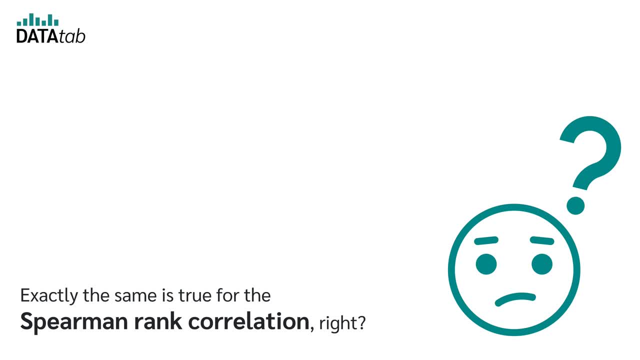 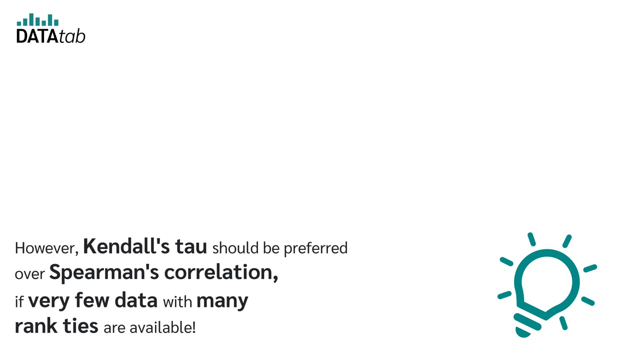 Exactly the same is true for the Spearman rank correlation. right, That's right. Kendall's tau is very similar to Spearman's rank correlation coefficient. However, Kendall's tau should be preferred over Spearman's correlation if very few data with many rank ties are available. 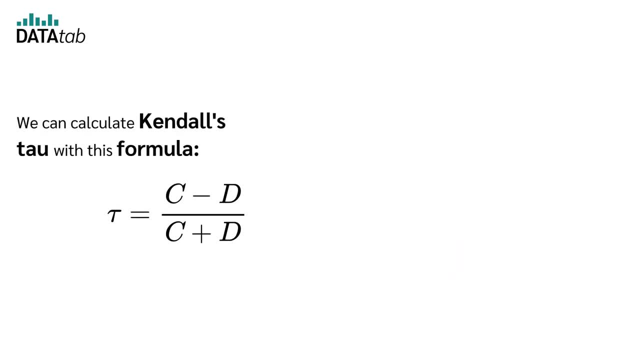 But how is Kendall's tau calculated? We can calculate Kendall's tau with this formula, where c is the number of concordant pairs and d is the number of discordant pairs. So we can calculate Kendall's tau with this formula, where c is the number of concordant pairs and d is the number of discordant pairs. 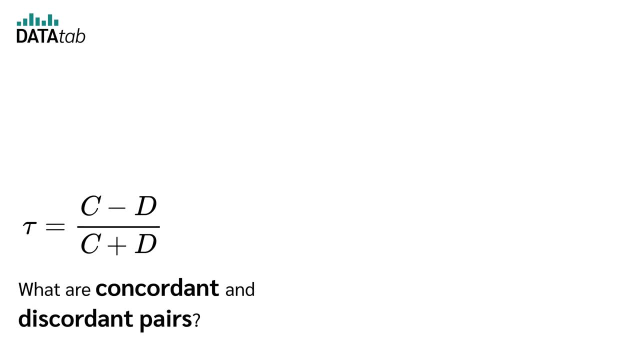 So we can calculate Kendall's tau with this formula, where c is the number of concordant pairs and d is the number of discordant pairs. What are concordant and discordant pairs? We will now go through this with an example. 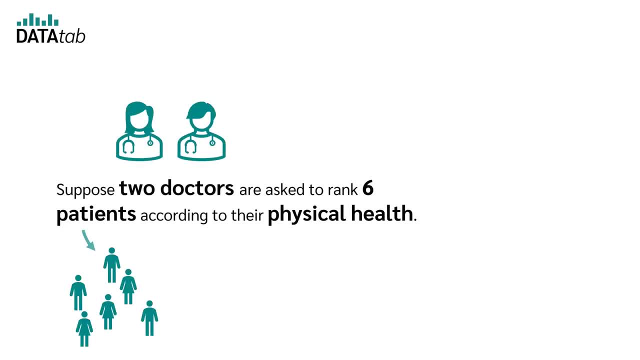 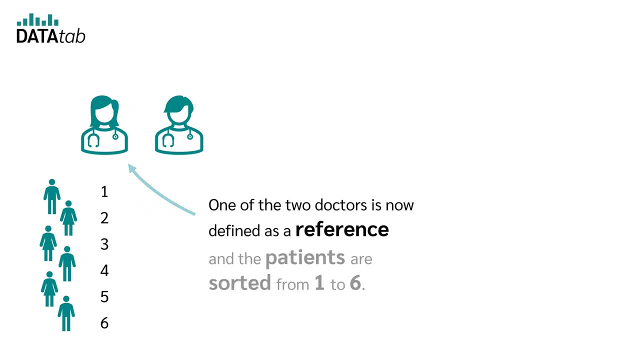 Suppose two doctors are asked to rank six patients according to their physical health. One of the two doctors is now defined as a reference and the patients are sorted from one to six. Now the sorted ranks are matched with the ranks of the other doctor, Eg. 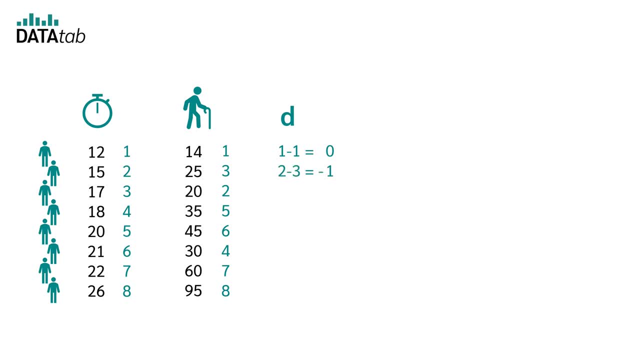 1 is equal to 0, 2 minus 3 is minus 1, 3 minus 2 is 1, and so on. Now we square the individual Ds and add them all up, So the sum of Di squared is 8.. 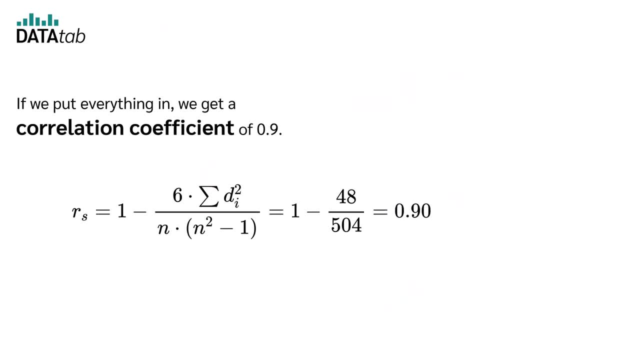 N, which is the number of people, is 8.. If you put everything in, we get a correlation coefficient of 0.9.. Just like the Pearson correlation coefficient R, Spearman correlation coefficient Rn S also varies between minus 1 and 1.. 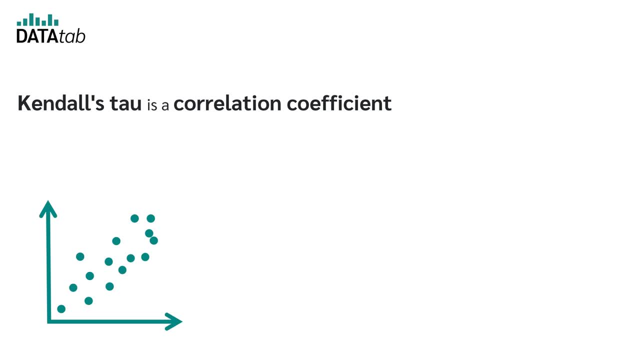 Let's continue with Kendall's tau. Kendall's tau is a correlation coefficient and is thus a measure of the relationship between two variables. But what is the difference between Pearson correlation and Kendall's rank correlation? In contrast to Pearson correlation, Kendall's rank correlation is a non-parametric test procedure. 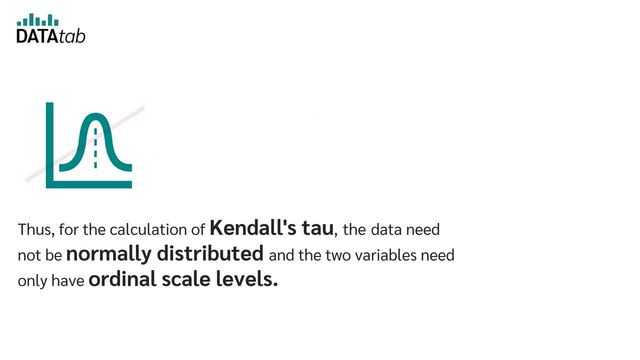 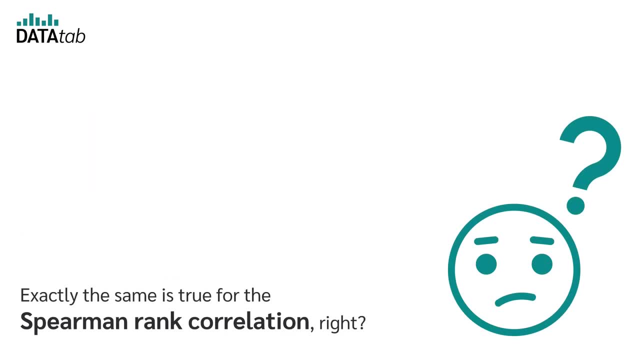 Thus, for the calculation of Kendall's tau, the data need not be normally distributed and the variables need only have ordinal scale levels. Exactly the same is true for the Spearman rank correlation. right, That's right. Kendall's tau is very similar to Spearman's rank correlation coefficient. 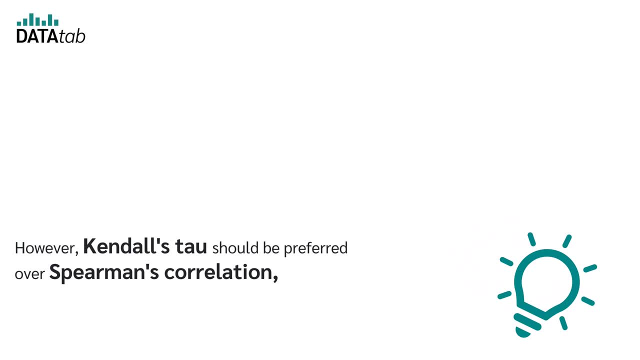 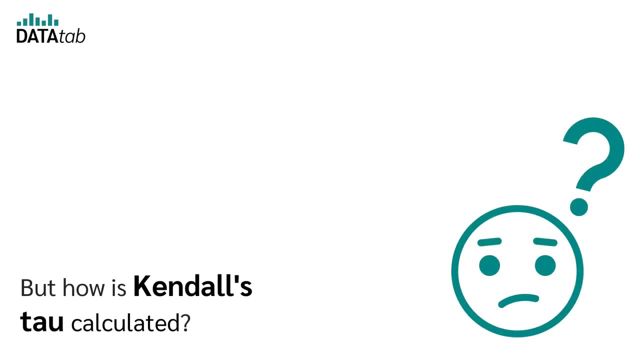 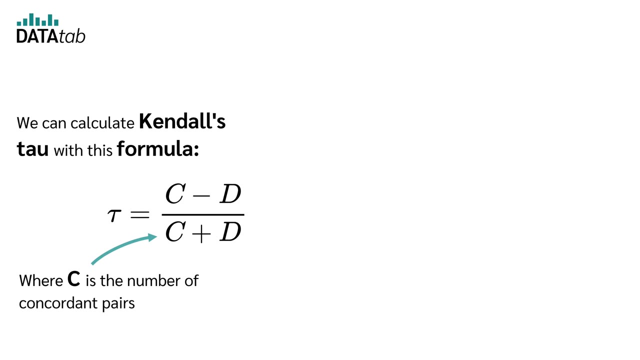 However, Kendall's tau should be preferred over Spearman's correlation if very few data with many rank ties are available. But how is Kendall's tau related to Spearman's rank correlation? We can calculate Kendall's tau with this formula, where C is the number of concordant pairs and D is the number of discordant pairs. 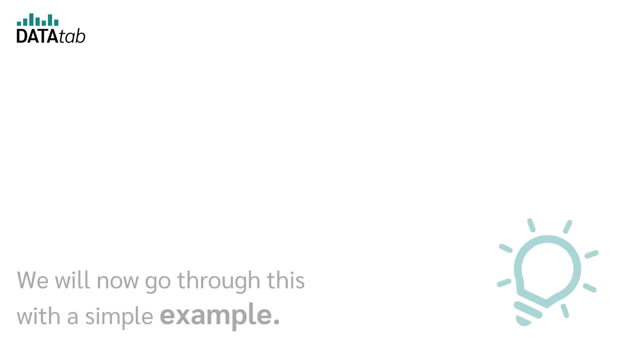 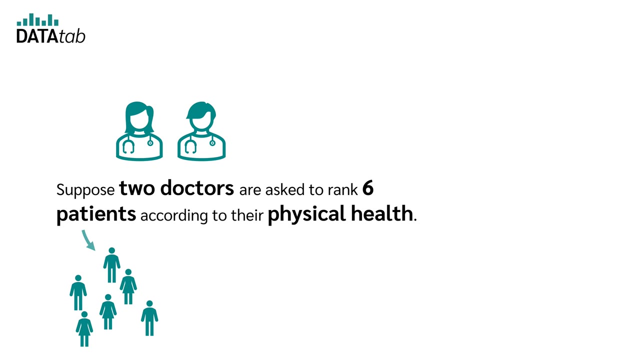 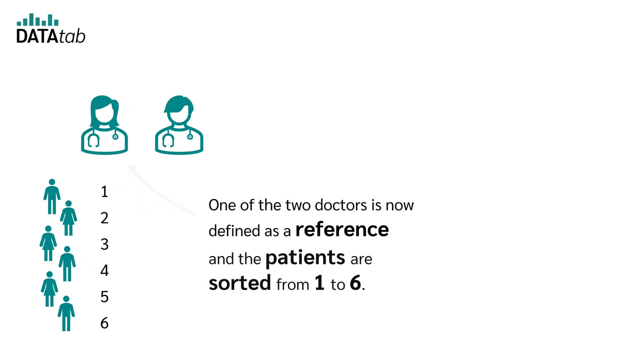 What are concordant and discordant pairs. We will now go through this with an example. Suppose two doctors are asked to rank six patients according to their physical health. One of the two doctors is now defined as a reference and the patient's rank is the number of patients according to their physical health. 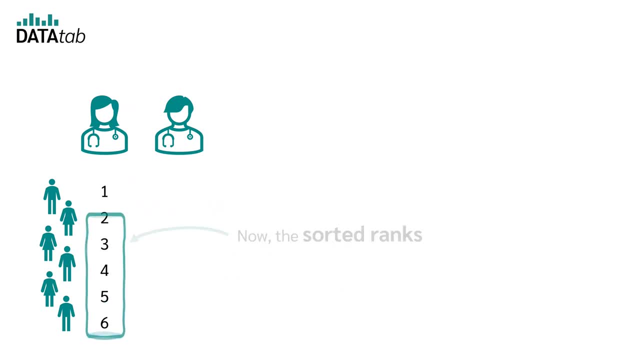 The patients are sorted from one to six. Now the sorted ranks are matched with the ranks of the other doctor, Eg, the patient who is in third place with the reference doctor is in fourth place with the other doctor Now using Kendall's tau, we want to know if there is a correlation. 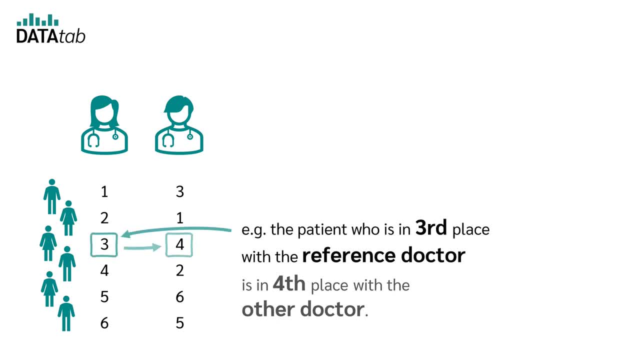 The patient who is in third place with the reference doctor is in fourth place with the other doctor Now using Kendall's tau. we want to know if there is a correlation between the two rankings For the calculation of Kendall's tau. we only need these ranks. 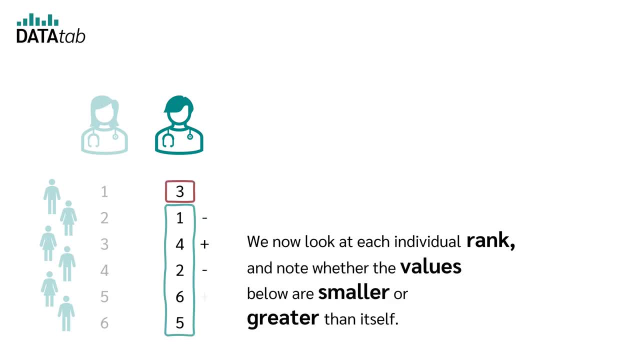 We now look at each individual rank and note whether the values below are smaller or greater than itself. So we start at the first rank. We now look at each individual rank and note whether the values below are smaller or greater than itself. We now look at each individual rank and note whether the values below are smaller or greater than itself. 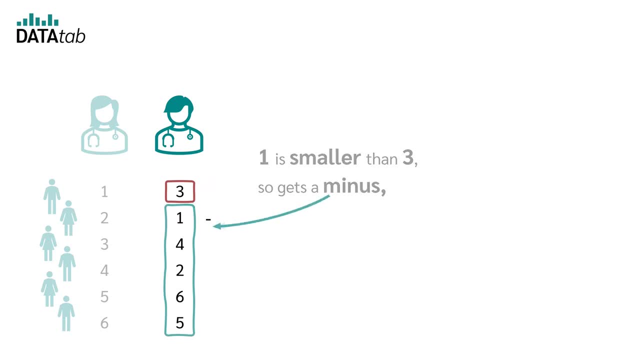 So we start at the first rank, 3.. 1 is smaller than 3, so gets a minus. 4 is greater, so gets a plus. 2 is smaller, so it gets a minus. 6 is greater, so it gets a plus. 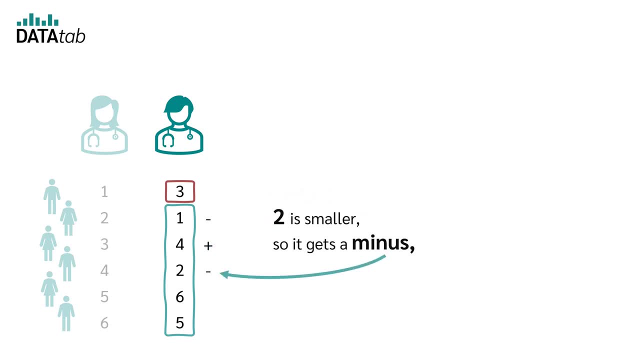 And 5 is also greater, so it also gets a plus. Now we do the same for 1.. Here, of course, each subsequent rank is greater than 1.. So we have a plus everywhere. At rank 4,, 2 is smaller and 6 is greater. 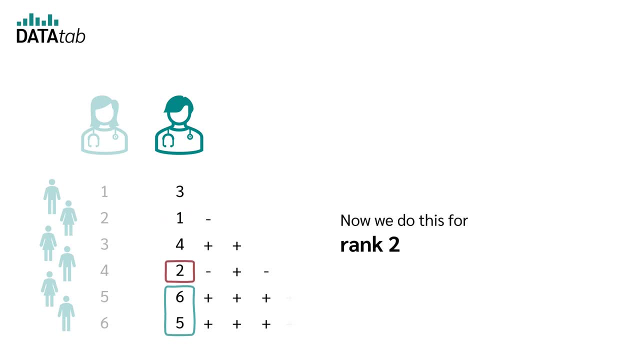 And 6 and 5 are greater. Now we do this for rank 2 and rank 6.. Then we can easily calculate the number of concordant and discordant pairs. We get the number of concordant pairs by counting all the plus. 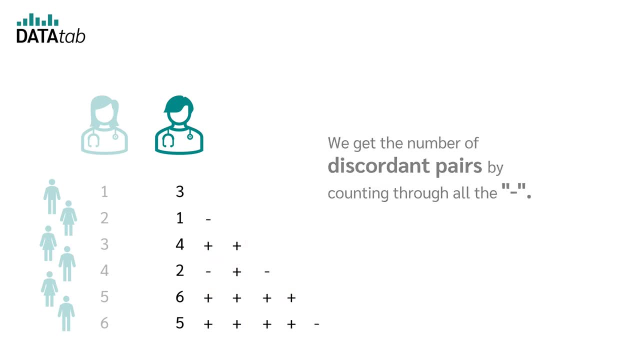 In our example, we have 11 plus in total. We get the number of discordant pairs by counting through all the minus. In our example, we have a total of 4 minus. So we get the number of discordant pairs by counting through all the minus. 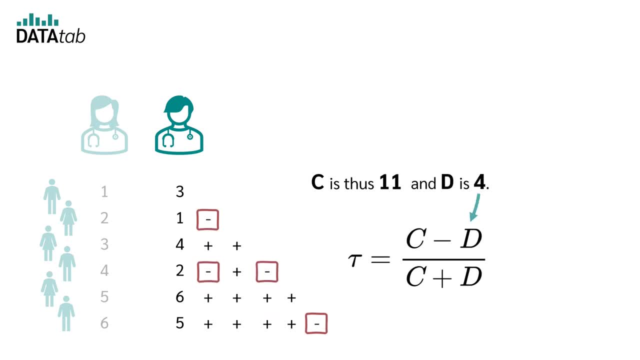 So we have a total of 4 minus. We get the number of concordant pairs by counting through all the minus. And next we have the number of concordant pairs by counting through all the plus. C is thus 11 and d is 4.. 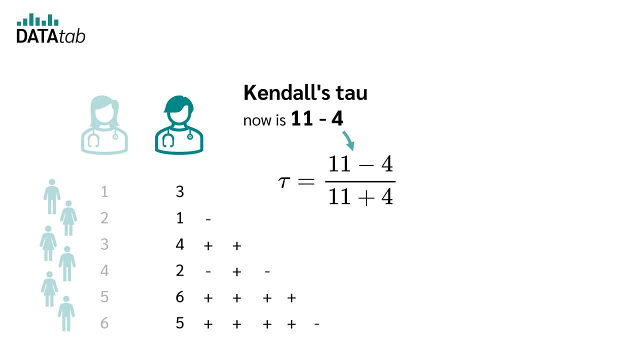 C is thus 11 and d is 4.. Candlestow now is 11 minus 4 divided by 11 plus 4.. And we get a Candlestow of 0.47.. We get an alternative formula for Candlestow herewith. 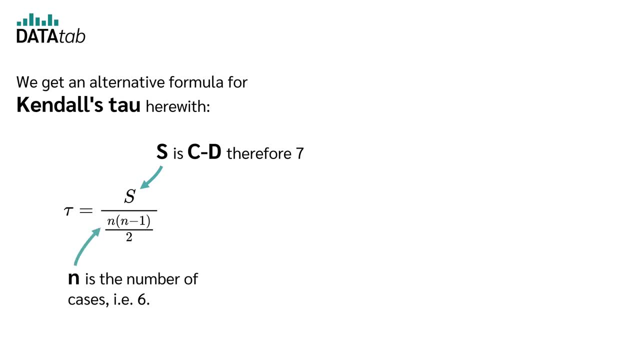 s is c minus d, therefore 7, and n is the number of cases, ie 6.. If we insert everything, we also get 7 divided by 6.. There we have it. Let's continue our proof by 15.. Just like the Pearson correlation coefficient r, Kendall's tau also varies. 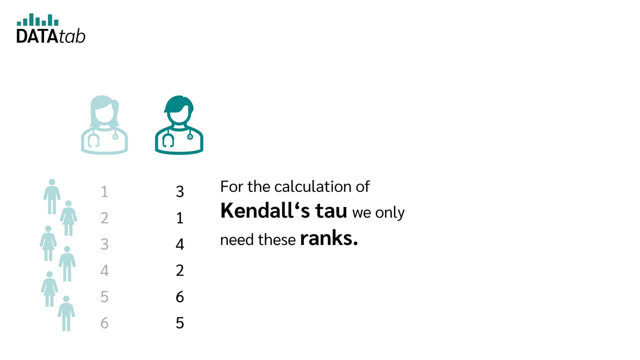 between the two rankings. For the calculation of Kendall's tau we only need these ranks. We now look at each individual rank and note whether the values below are smaller or greater than itself. So we start at the first rank, 3.. 1 is smaller than 3, so gets a minus. 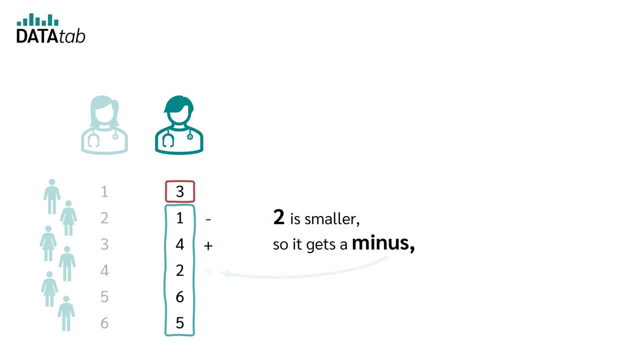 4 is greater, so gets a plus. 2 is smaller, so it gets a minus. 6 is greater, so it gets a plus. And 5 is also greater, so it also gets a plus. Now we do the same for 1.. 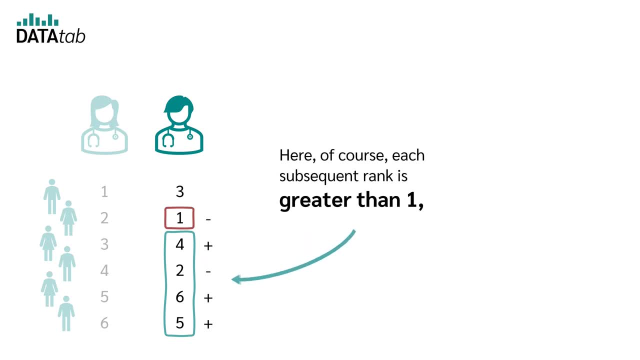 Here, of course, each subsequent rank is greater than 1.. So we have a plus everywhere. At rank 4,, 2 is smaller and 6 and 5 are greater. Now we do this for rank 2 and rank 6.. 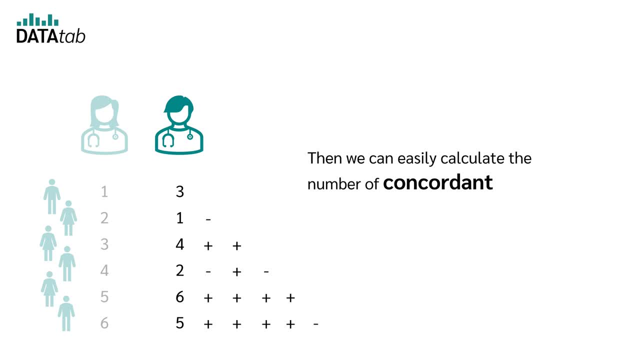 Then we can easily calculate the number of concordant and discordant pairs. We get the number of concordant pairs by counting all the plus. In our example we have 11 plus in total. We get the number of discordant pairs by counting through all the minus In our 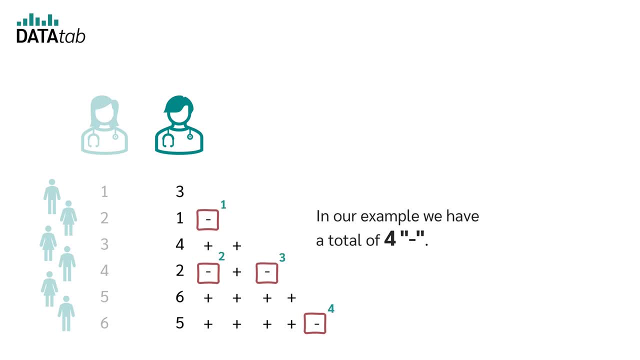 example, we have a total of 4 minus C is thus 11 and D is 4.. Kendall's tau now is 11 minus 4 divided by 11 plus 4, and we get a Kendall's tau of 0.47.. 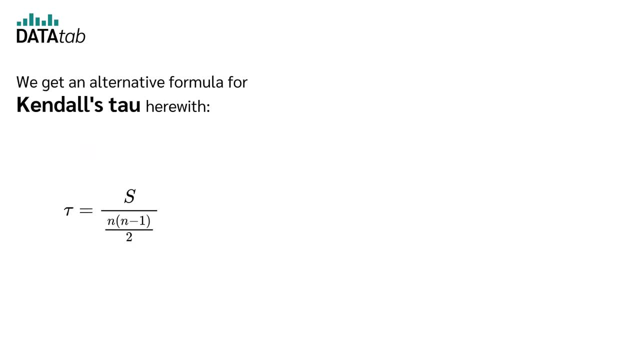 And we get an alternative formula for Kendall's tau, here with S yes, because аств lice alone will yield the answer C plus Rz. Here we get 4 cuentals düşen mal eine also, Also餅 이야기. 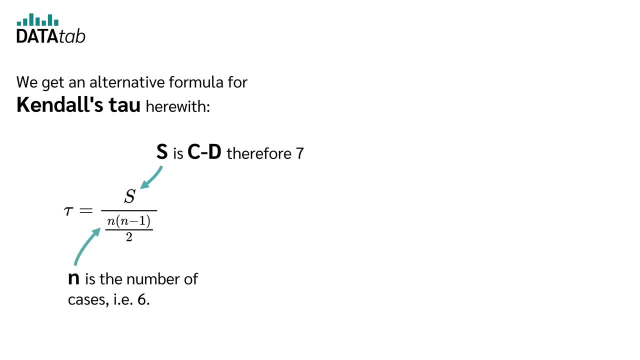 is c minus d, therefore 7, n is the number of cases, ie 6.. If we insert everything, we also get 7 divided by 15.. Just like the Pearson correlation coefficient r, Kendall's tau also varies between minus 1 and plus 1.. We have again calculated the correlation coefficient. 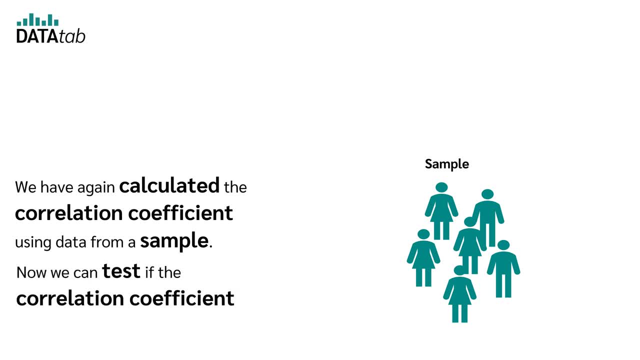 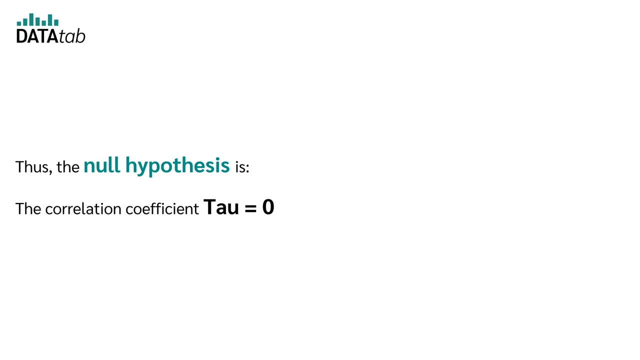 using data from a sample. Now we can test if the correlation coefficient is significantly different from 0. Thus the null hypothesis is the correlation coefficient. tau is equal to 0, there is no relationship. And the alternative hypothesis is the correlation coefficient. 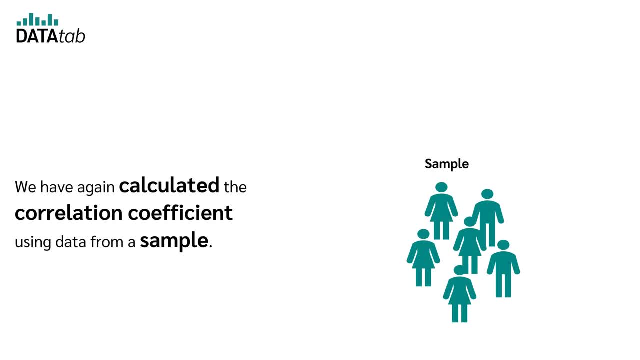 between minus 1 and plus 1.. We have again calculated the correlation coefficient using data from a sample. Now we can test if the correlation coefficient is significantly different from zero. Thus the null hypothesis is the correlation coefficient. tau is equal to zero. 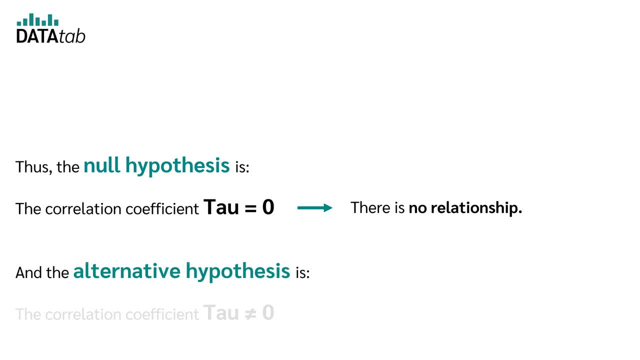 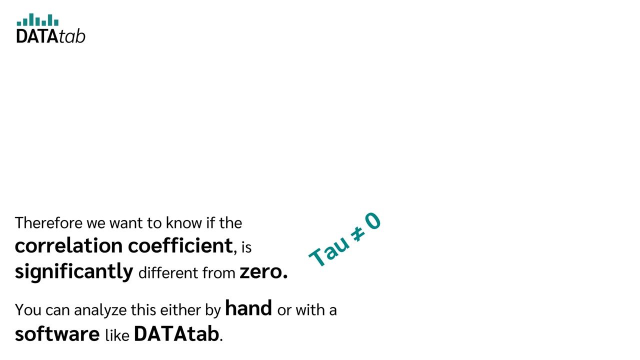 there is no relationship. And the alternative hypothesis is the correlation coefficient tau is unequal to zero. there is a relationship. Therefore, we want to know if the correlation coefficient is significantly different from zero. You can analyze this either by hand or with a software like DataTab. For the calculation by hand, we can use the. 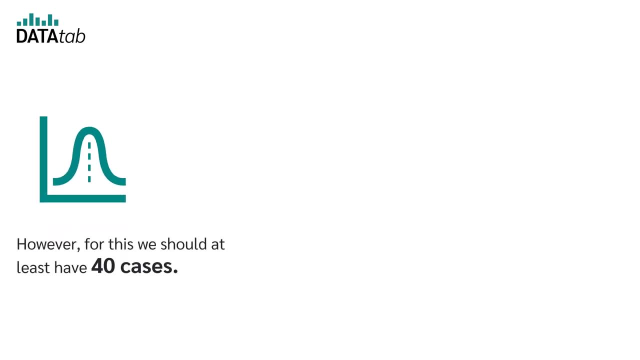 set distribution as an approximation. However, for this we should at least have 40 cases, so the 6 cases from our example are actually too few. We get the set value with this formula. Here we have tau and n is the number of cases. This brings us to the last correlation analysis. 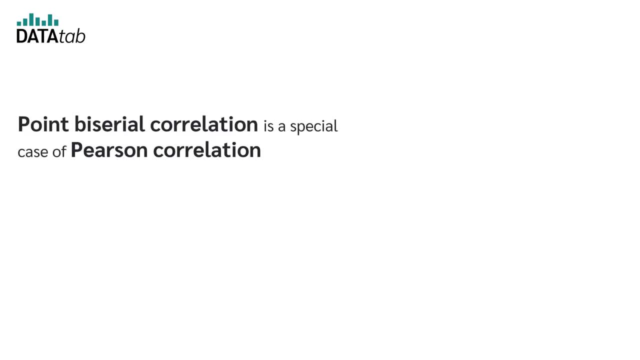 the point by zero correlation. Point by zero correlation is a special case of Pearson correlation and examines the relationship between a dichotomous variable and the metric variable. What is a dichotomous variable? It is a dichotomous variable that is equal to the number of cases. 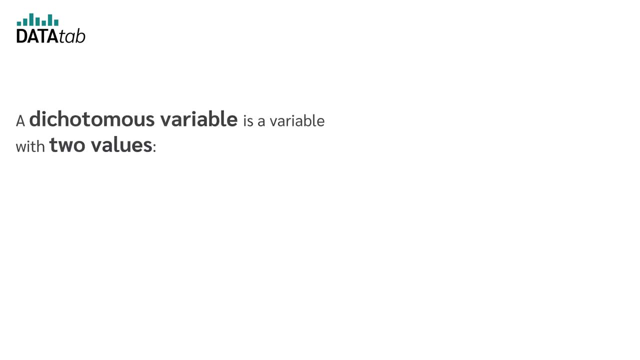 So what is a dichotomous variable? What is a metric variable? A dichotomous variable is a variable with two values, for example, gender, with male and female, or smoking status, with smoker and non-smoker. A metric variable is, for example, the weight of a person, the. 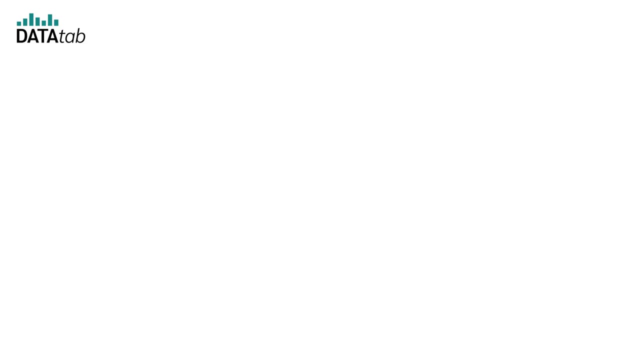 salary of a person or the electricity consumption. So if we have a dichotomous variable and a metric variable and we want to know if there is a dichotomous variable, what is a metric variable? The dichotomous variable is a variable. 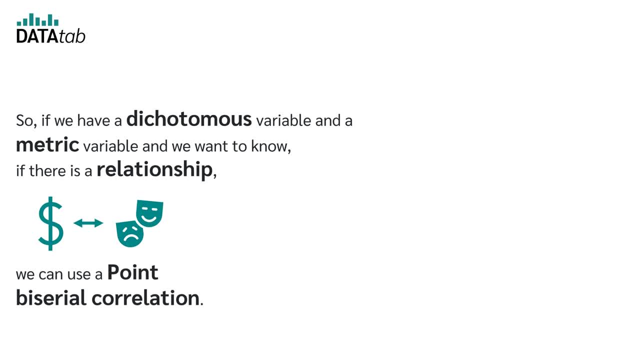 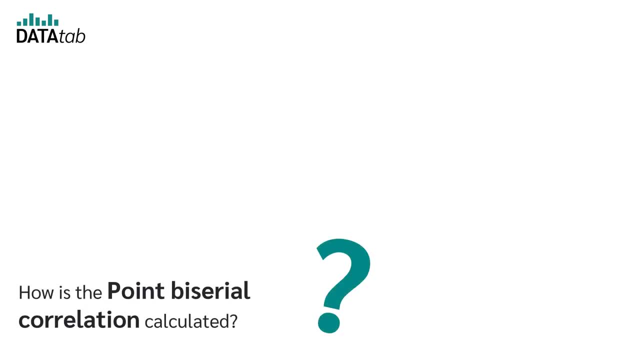 of a person whose entire life superimposed on pure mole in order to take real cases, While the Carmenstam child is superimposed on pure mole in order to take real cases. What if the function of Holiday ==== Well, in a relationship we can use a point by zero correlation? Of course we need to. 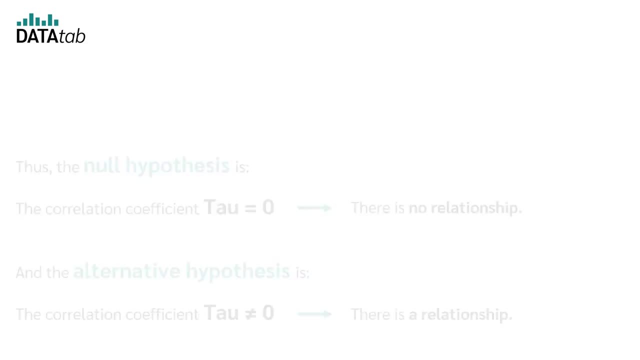 tau is unequal to 0, there is a relationship. Therefore, we want to know if the correlation coefficient is significantly different from 0. You can analyze this either by hand or with a software like DataTab. For the calculation by hand, we can use the set distribution as an approximation. 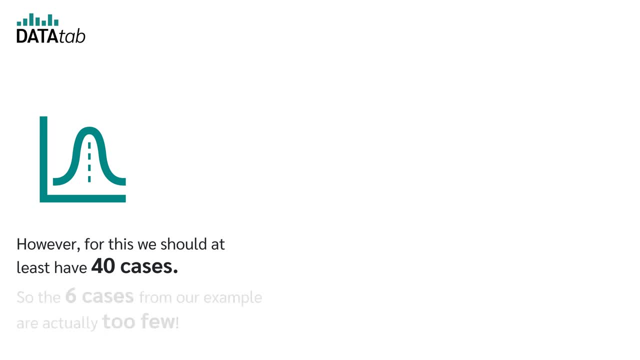 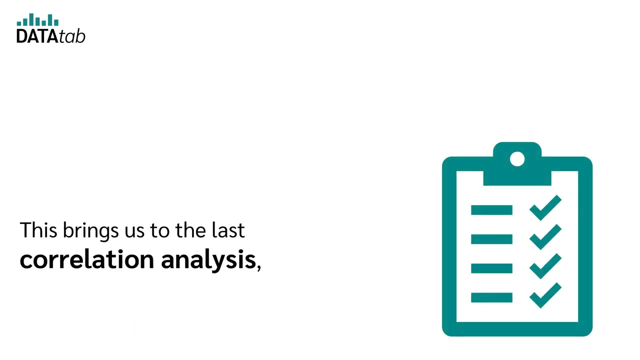 However, for this we should at least have 40 cases. So the 6 cases from our example are actually too few. We get the set value with this formula. Here we have tau and n is the number of cases. This brings us to the last correlation analysis, the point-by-zerial correlation. 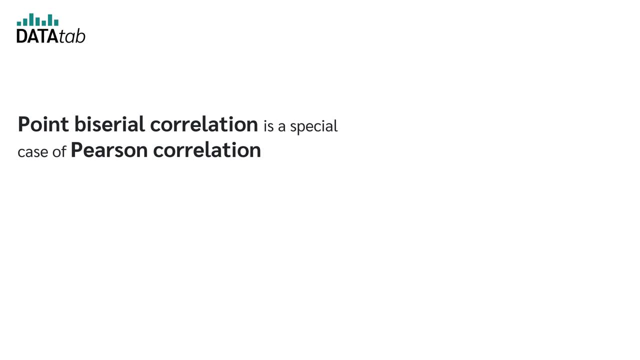 Point-by-zerial correlation is a special case of Pearson correlation and examines the relationship between a dichotomous variable and a metric variable. What is a dichotomous variable and what is a metric variable? A dichotomous variable is a variable with two values, for example gender with male. 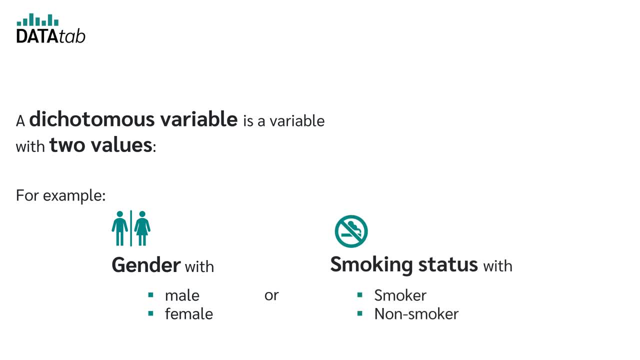 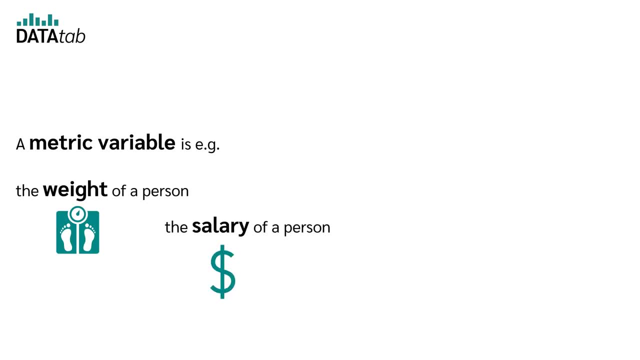 and female Or smoking status. A metric variable is, for example, the weight of a person, the salary of a person or the electricity consumption. So if we have a dichotomous variable and a metric variable and we want to know if there 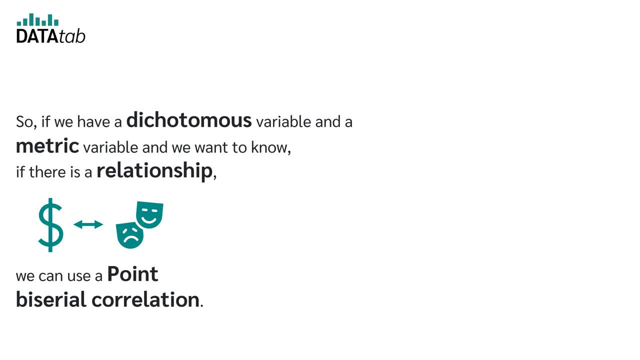 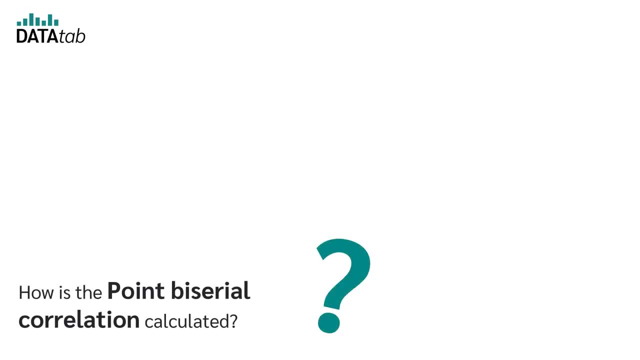 is a relationship, we can use a point-by-zerial correlation. Of course, we need to check the assumptions beforehand, but more about that later. How is the point-by-zerial correlation? As stated at the beginning, the point-by-zerial correlation is a special case of the Pearson. 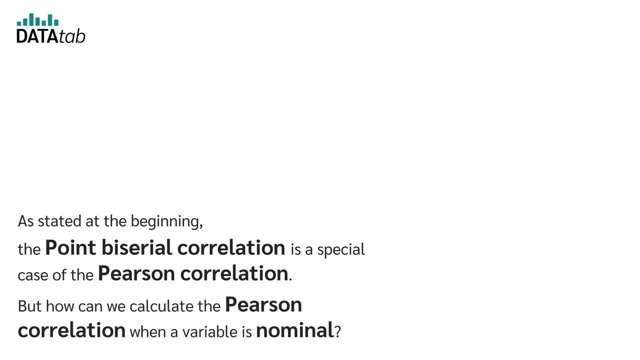 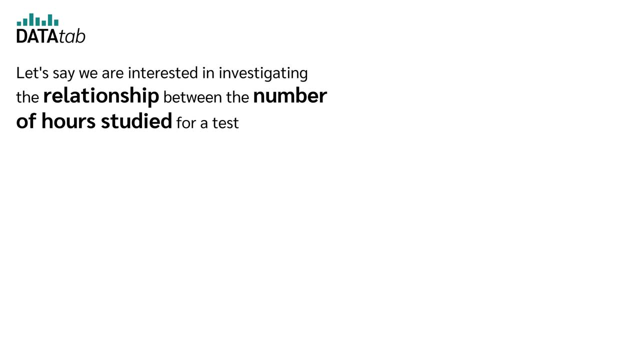 correlation. But how can we calculate the Pearson correlation when a variable is nominal? Let's look at this with an example. Let's say we are interested in investigating the relationship between the number of hours studied for a test and the test result passed failed. 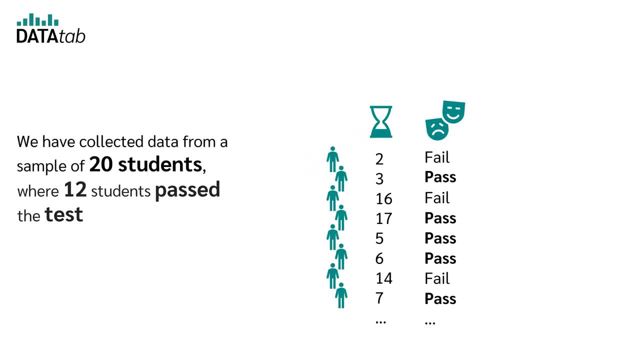 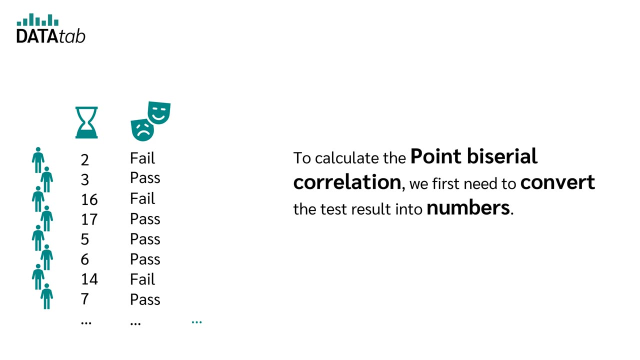 We've calculated data from a study. We have a sample of 20 students, where 12 students passed the test and 8 students failed. We have recorded the number of hours each student studied for the test. To calculate the point-by-zerial correlation, we first need to convert the test result into: 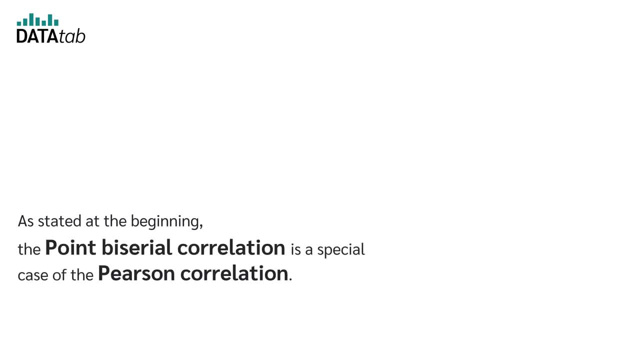 check the assumptions, But more about that later. How is the point by zero correlation calculated? As stated at the beginning, the point by zero correlation is a special case of the Pearson correlation. but how can we calculate the Pearson correlation when a variable is nominal? 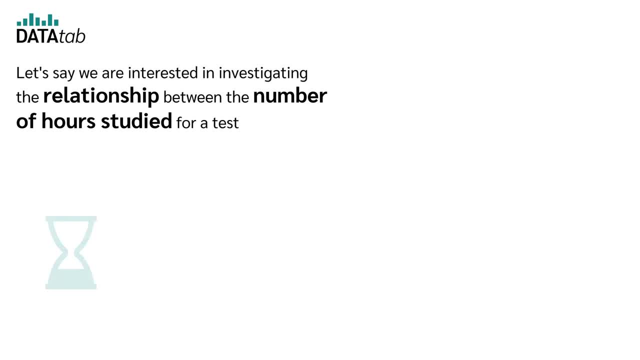 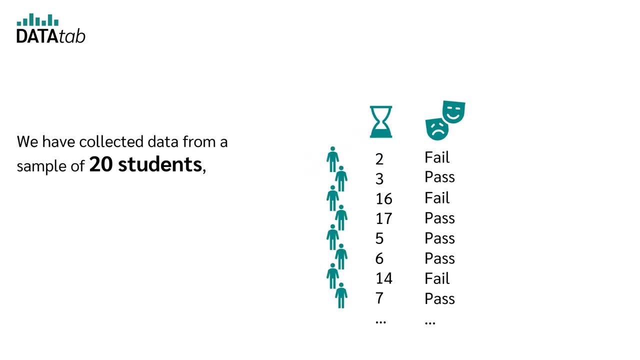 interested in investigating the relationship between the number of hours studied for a test and the test result passed-failed. We've calculated data from a sample of 20 students, where 12 students passed the test and 8 students failed. We have recorded the number of hours each student studied for the test. 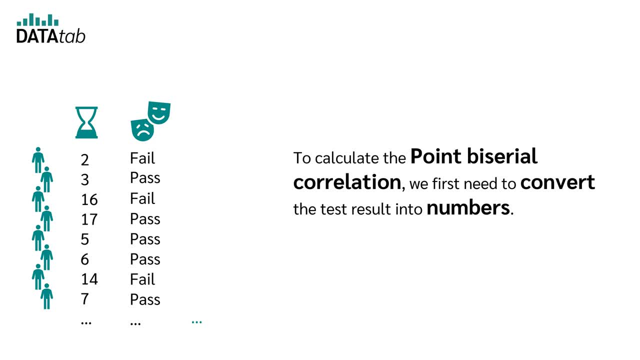 To calculate the point by zero correlation, we first need to convert the test result into numbers. We can assign a score of one to students who passed the test and a score of zero to the students who failed the test. Now we can either calculate the Pearson correlation of time and test result or we use the equation. 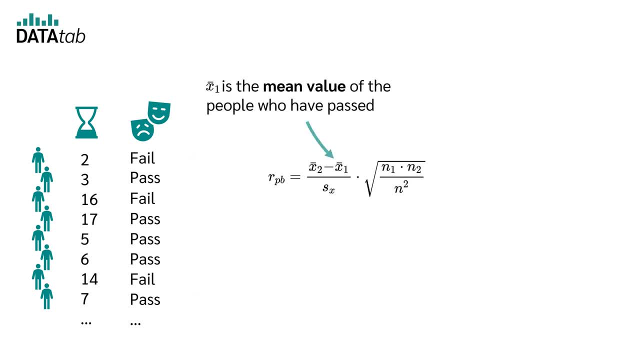 for the point by zero correlation. x1' is the mean value of the people who have passed and x2' is the mean value of the people who failed. n1 is the number of people who passed and n2 the number of people who failed, and n is the total number. 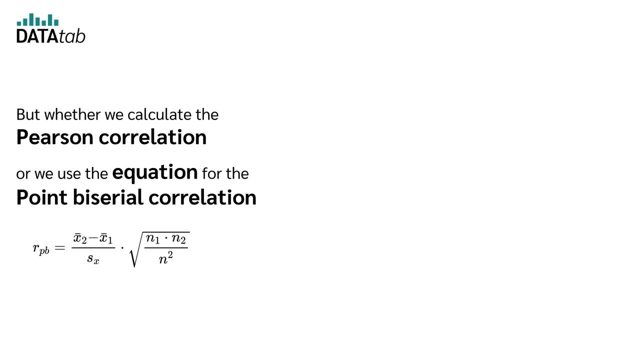 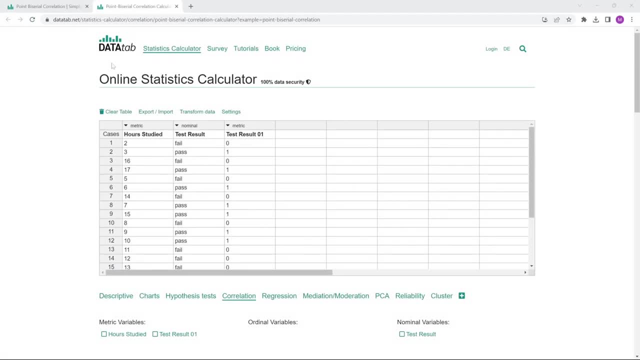 But whether we calculate the Pearson correlation or we use the equation for the point-by-zero correlation, we get the same result both times. Let's take a quick look at this in DataTab. Here we have the learning hours, the test result with passed and failed, and there the 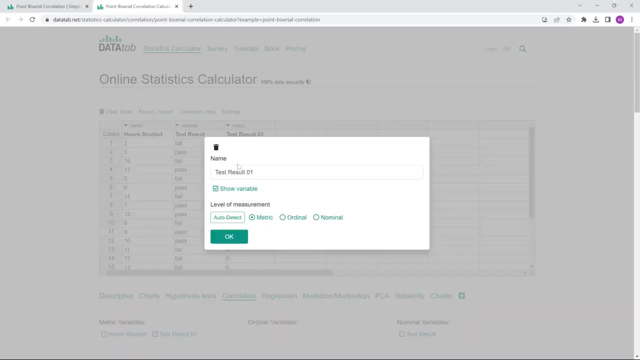 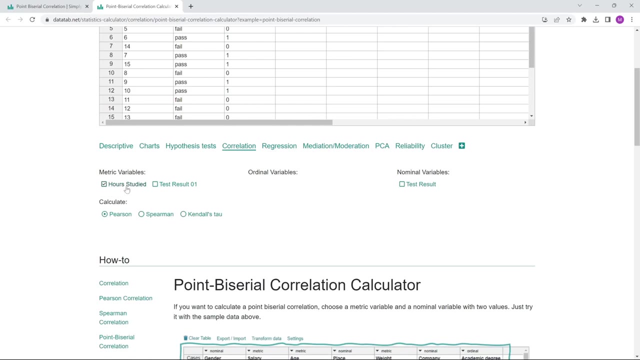 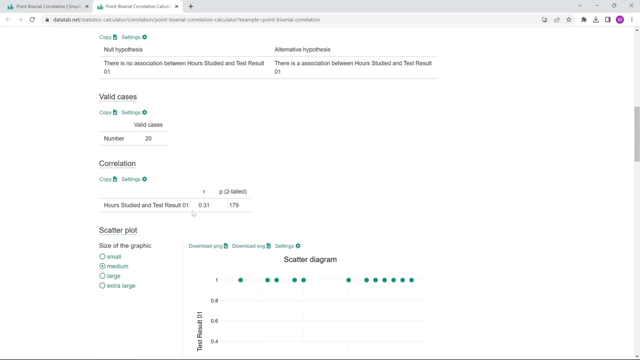 test result with zero and 1.. We define the test result with zero and 1 as metric. If we now go to correlation and calculate the pierson correlation for these two variables, we get a correlation coefficient of 0.31.. If we calculate the point-by-zero correlation for learning hours and expressions we get at about identical numbers, which are then multiplied each time and Kappa is their value, and I am not going to see key numbers over and over Now. I am going to look at this. So the reference data in my example is already on the倉lsci liter and kappa equals 0.81, which also 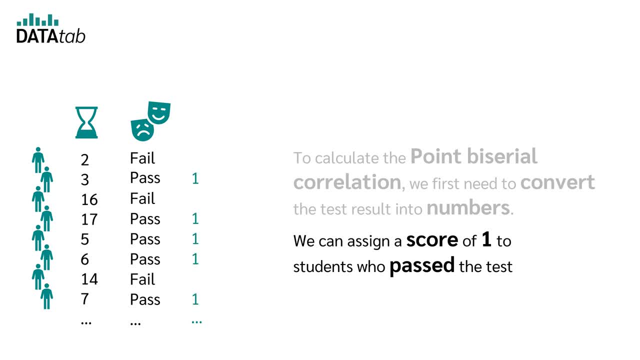 numbers. We can assign a score of 1 to students who passed the test and a score of 0 to students who failed the test. Now we can either calculate the Pearson correlation- We can use the equation of time and test result- Or we use the equation for the point-by-zerial correlation. 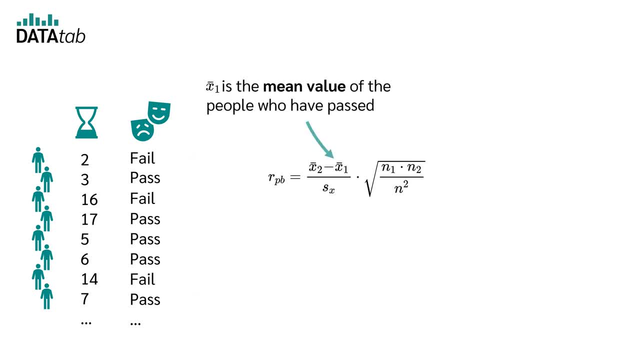 x1' is the mean value of the people who have passed and x2' is the mean value of the people who failed. n1 is the number of people who passed and n2 the number of people who failed, And n is the total number. 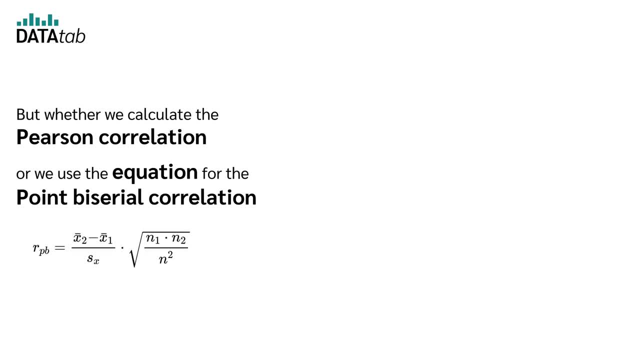 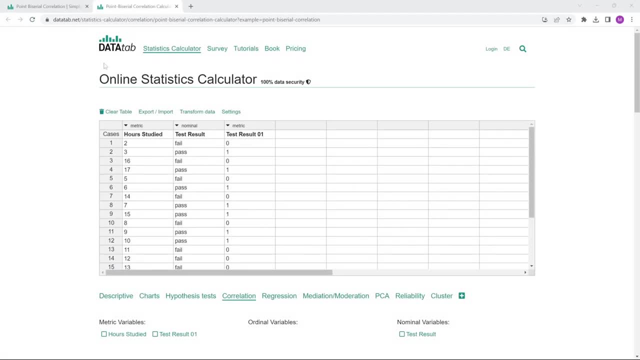 But whether we calculate the Pearson correlation or we use the equation for the point-by-zerial correlation, we get the same result both times. Let's take a quick look at this in DataTab. Here we have the learning hours, the test result with passed and failed, and there the 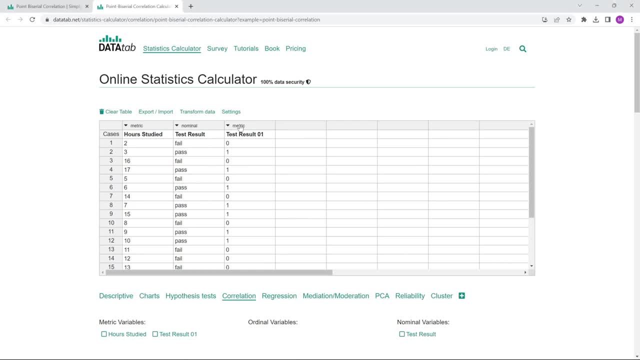 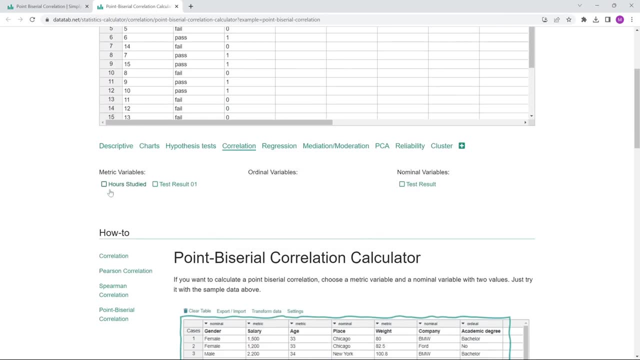 test result with 0 and 1.. We define the test result with 0 and 1 as metric. If we now go to correlation and calculate the Pearson correlation for these two variables, we get a correlation coefficient of 0 and 1.. 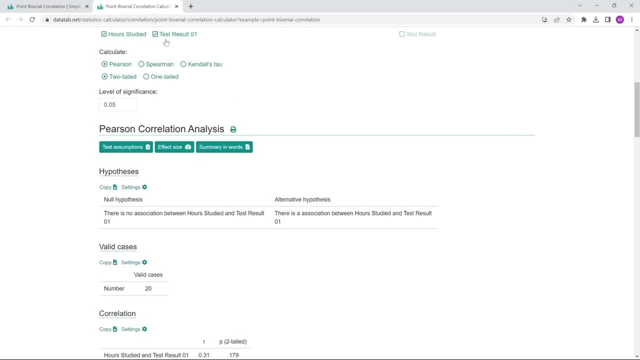 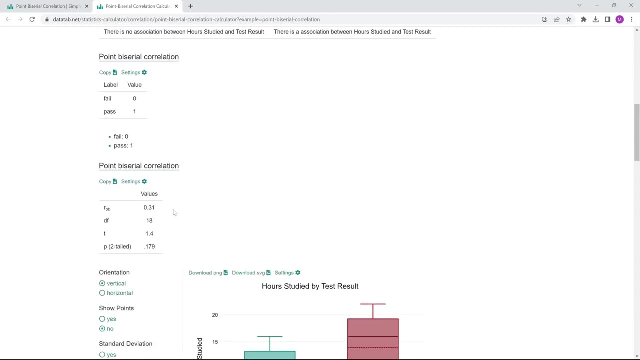 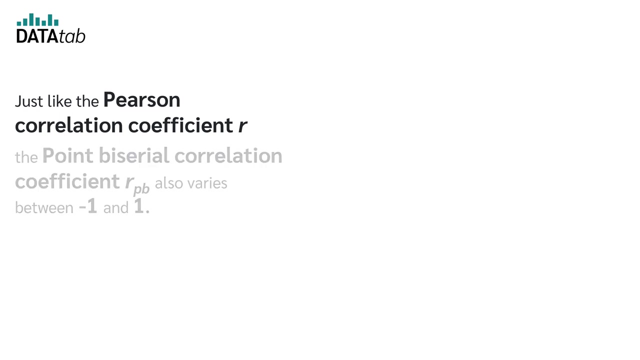 Let's take a look at this in DataTab. If we calculate the point-by-zerial correlation for learning hours and the exam result with passed and failed, we also get a correlation of 0.31.. Just like the Pearson correlation coefficient r, the point-by-zerial correlation coefficient. 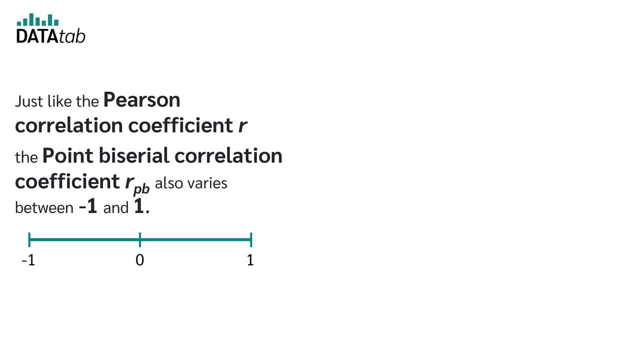 rpb also varies between minus 1 and 1.. If we have a coefficient between minus 1 and less than 1, there is a negative correlation, Thus a negative relationship between the variables. If we have a coefficient between greater than 0 and 1, there is a positive correlation. 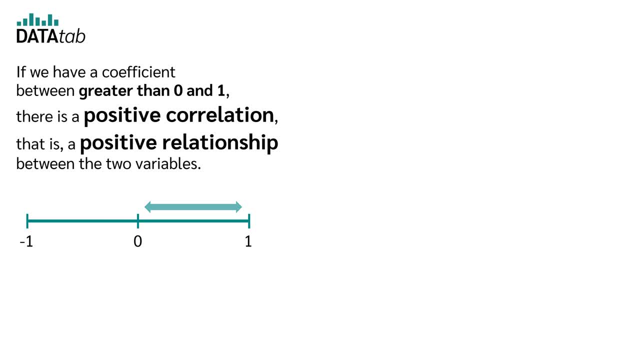 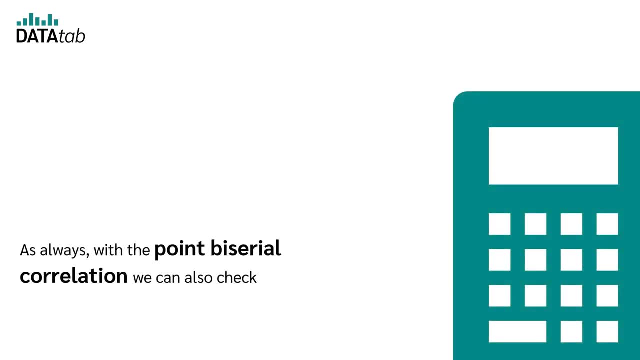 That is a positive relationship between the two variables. If the result is 0,, we have no correlation. As always, with the point-by-zerial correlation, we can also check whether the correlation coefficient is significantly different from 0. Thus the null has no correlation. 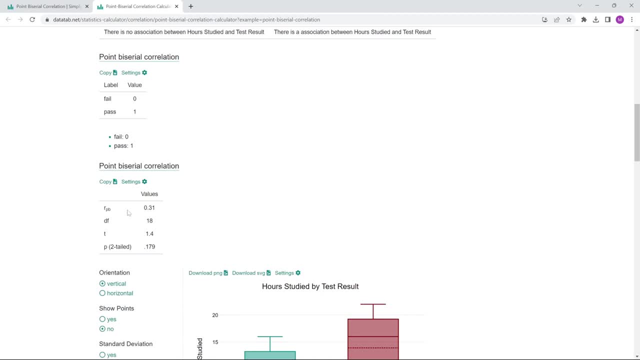 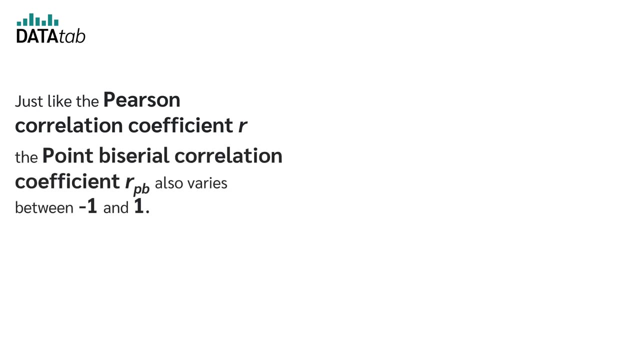 result: with passed and failed, we also get a correlation of 0.31.. Just like the Pearson correlation coefficient r, the point-by-zero correlation coefficient rpb also varies between minus 1 and 1.. If we have a coefficient between minus 1 and less than 1, there is a negative. 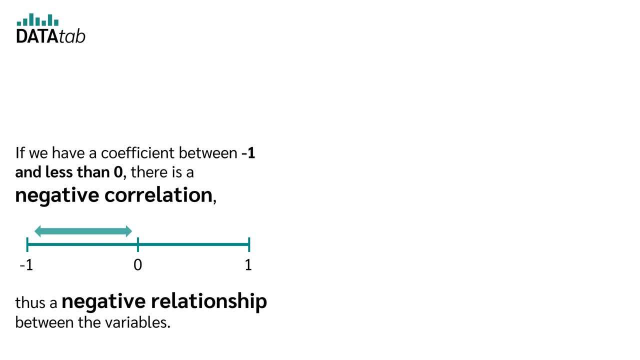 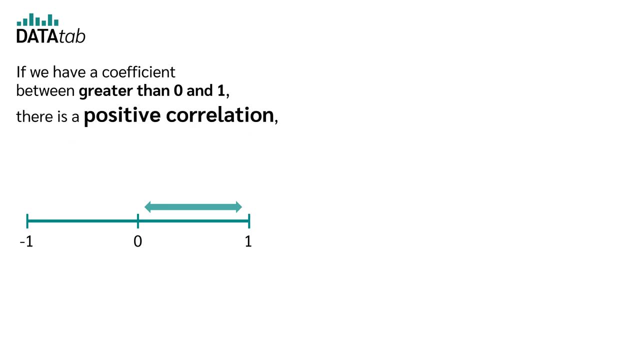 correlation, thus a negative relationship between the variables. If we have a coefficient between greater than zero and one, there is a positive correlation, that is, a positive relationship between the two variables. If the result is 0, we have no correlation, As always with the point. 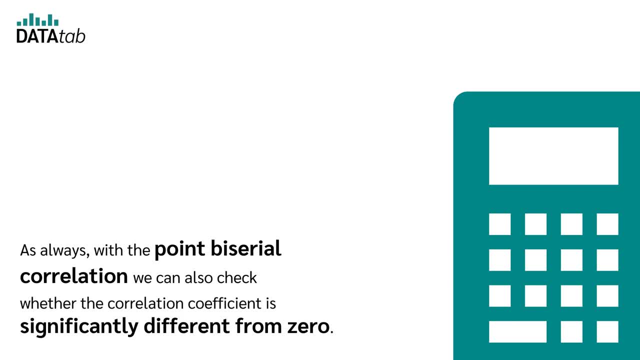 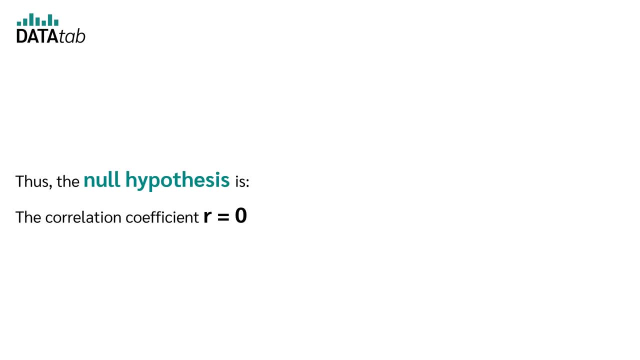 by zero correlation, we can also check whether the correlation coefficient is significantly different from 0. Thus the null hypothesis is: the correlation coefficient r is equal to 0, there is no relationship. And the alternative hypothesis is: the correlation coefficient r is unequal to zero. there is a relationship. 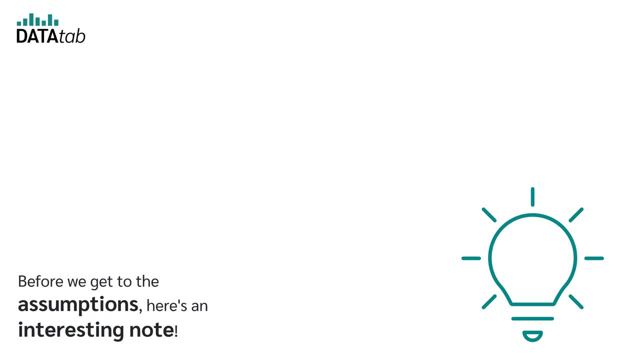 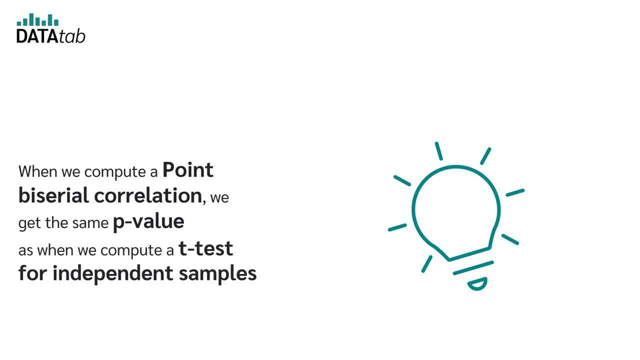 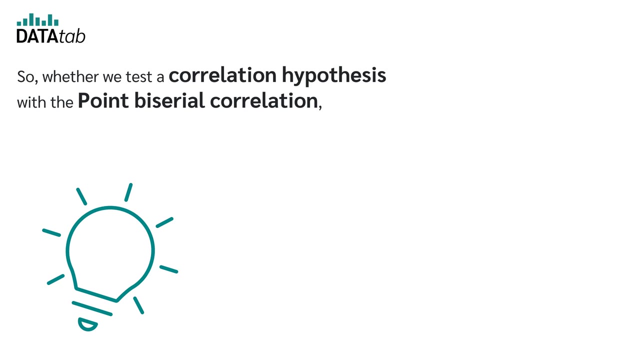 Before we get to the assumptions, here's an interesting note. When we compute a point-by-zero correlation, we get the same p-value as when we compute a t-test for independent samples for the same data. So whether we test a correlation hypothesis with the point-by-zero correlation, 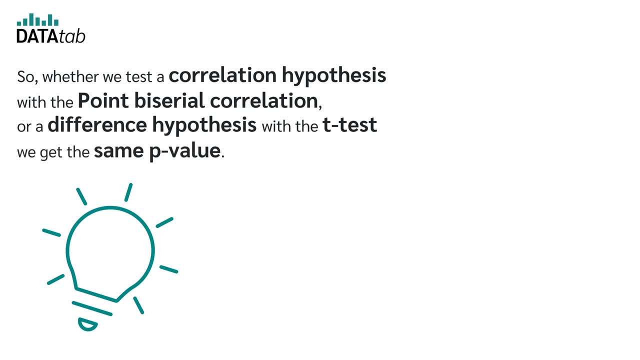 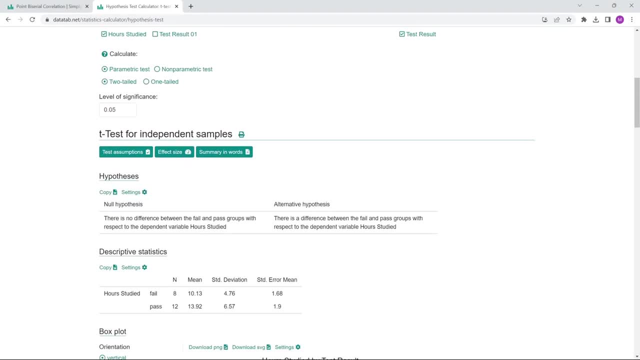 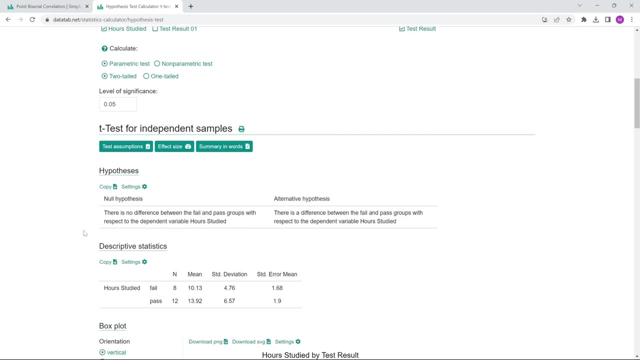 or a difference hypothesis. with the t-test, we get the same p-value. Now, if we compute a t-test in DataTab with these data and we have the null hypothesis, there is no difference between the groups failed and passed. in terms of the variable learning hours, we get a p-value. 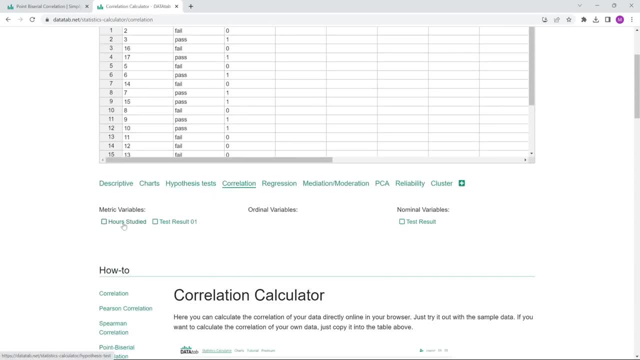 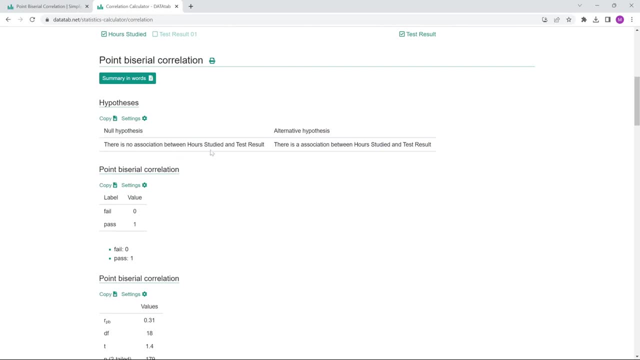 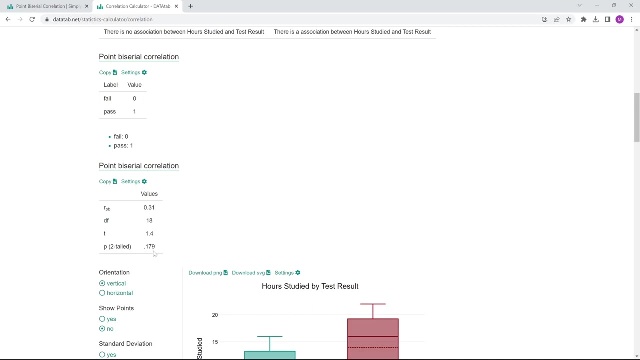 of 0.179.. And also, if we calculate a point-by-zero correlation and have the null hypothesis, there is no correlation. If we calculate a point-by-zero correlation between learning hours and test results, we get a p-value of 0.179.. In our example, the p-value is greater than 0.05, which is most. 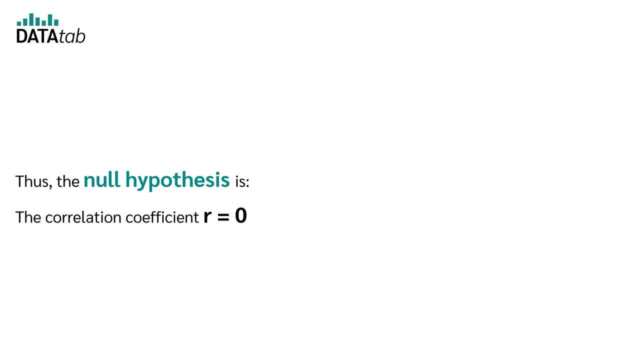 Let's take a look at this. The null hypothesis is the correlation coefficient r is equal to 0, there is no relationship. And the alternative hypothesis is the correlation coefficient r is unequal to 0, there is a relationship. Before we get to the assumptions, here's an interesting note. 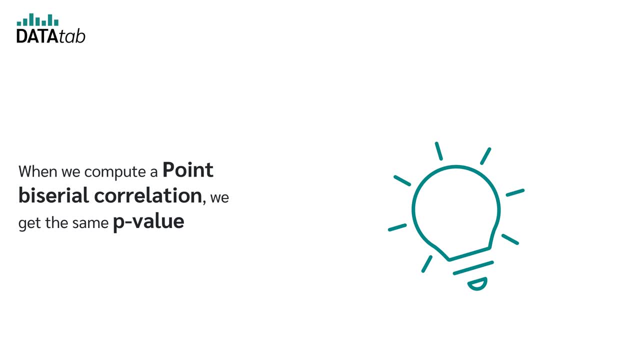 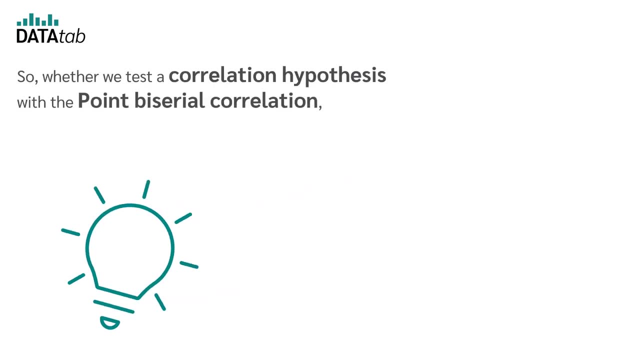 When we compute a point-by-zerial correlation, we get the same p-value as when we compute a t-test for independent samples for the same data. Let's take a look at this. So, whether we test a correlation hypothesis with the point-by-zerial correlation or a 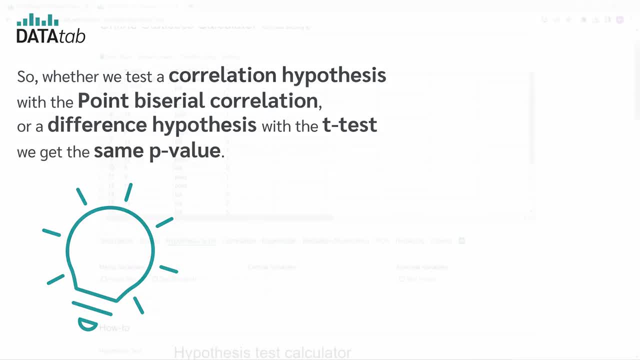 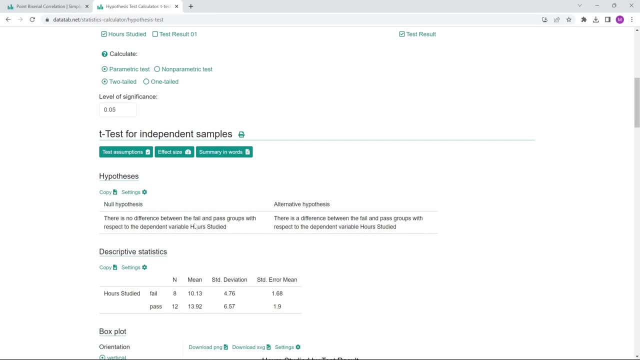 difference hypothesis. with the t-test we get the same p-value. Now if we compute a t-test in data-tab with these data and we have the null hypothesis, there is no difference between the groups failed and passed in terms of the variable. 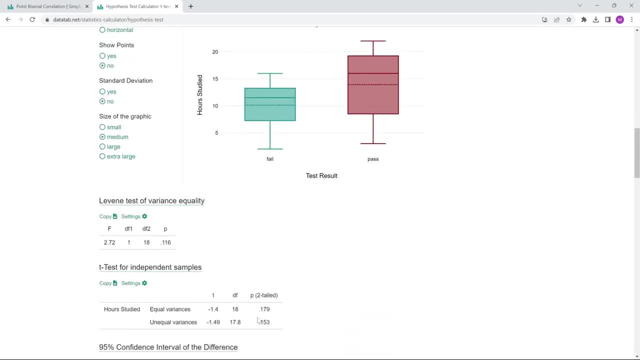 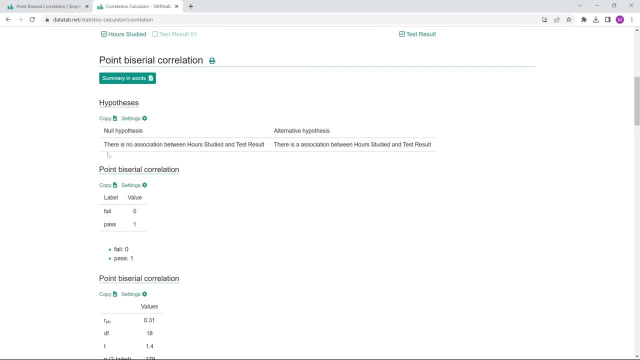 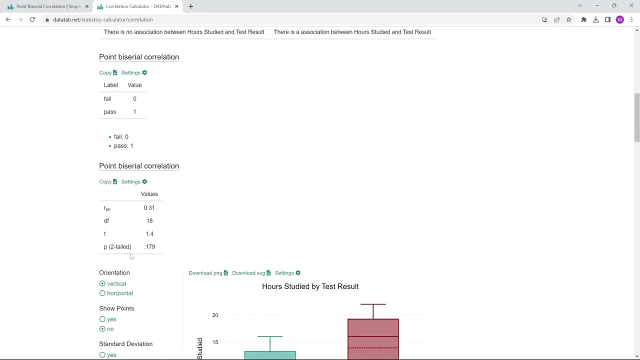 learning hours, we get a p-value of 0.179.. And also, if we calculate a point-by-zerial correlation and have the null hypothesis, there is no correlation between learning hours and test results- we get a p-value of 0.179.. 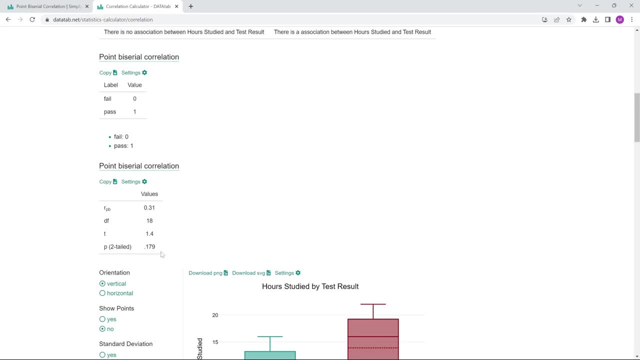 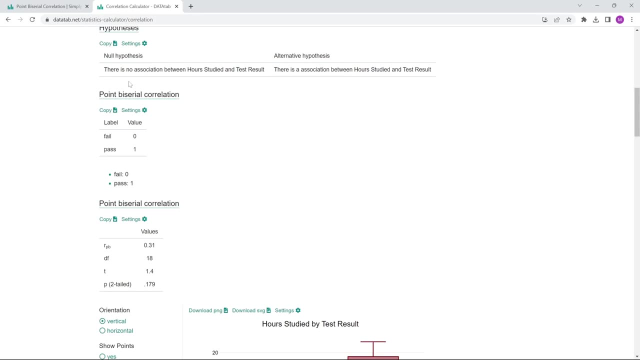 In our example, the p-value is greater than 0.05, which is most often used as a significance level, and thus the null hypothesis is not rejected. But what about the assumptions for a point-by-zerial correlation? Let's take a look at the assumptions for a point-by-zerial correlation. 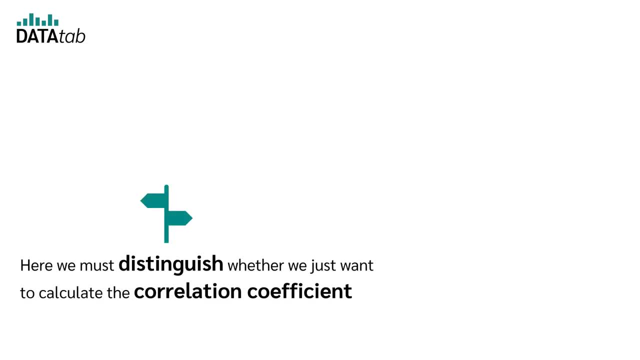 Let's take a look at the assumptions for a point-by-zerial correlation. Let's take a look at the assumptions for a point-by-zerial correlation. Here we must distinguish whether we just want to calculate the correlation coefficient or whether we want to test a hypothesis. 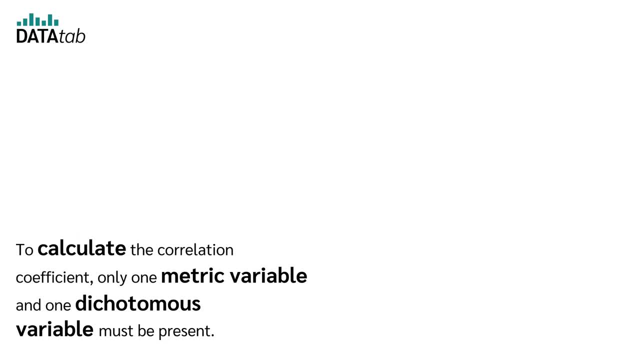 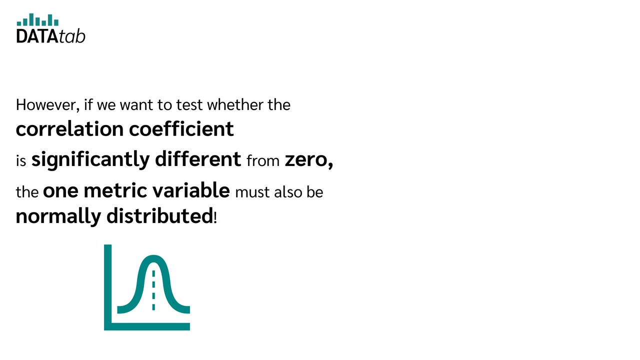 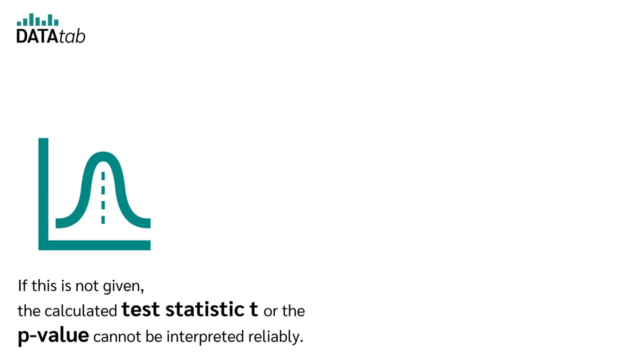 To calculate the correlation coefficient, only one metric variable and one dichotomous variable must be present. However, if we want to test whether the correlation coefficient is significantly different from zero, the one metric variable must also be normally distributed. If this is not given, the calculated test statistic t or the p-value cannot be interpreted. 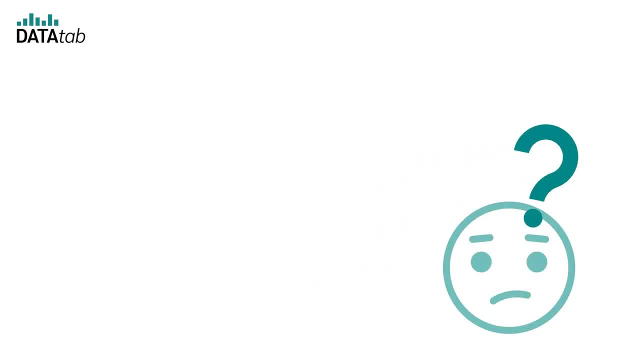 reliably. This brings us to the last question: What is causality And what is the difference between causality and correlation? Causality is the relationship between a cause and an effect. In a causal relationship, we have a cause and a resultant effect. 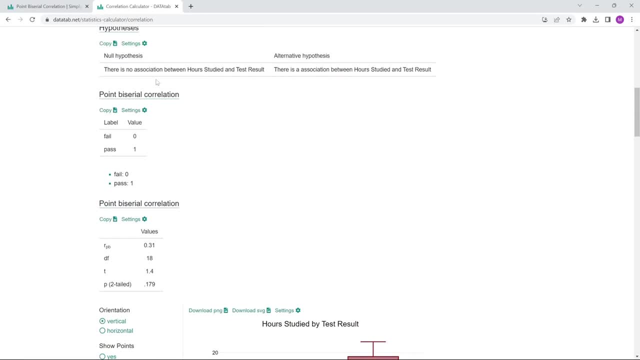 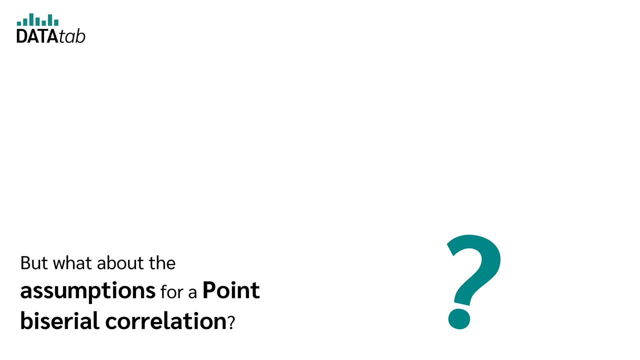 often used as a significance level, and thus the null hypothesis is not rejected. But what about the assumptions for a point-by-zero correlation? Here we must distinguish whether we just want to calculate the correlation coefficient or whether we want to test a hypothesis To calculate the correlation coefficient only. 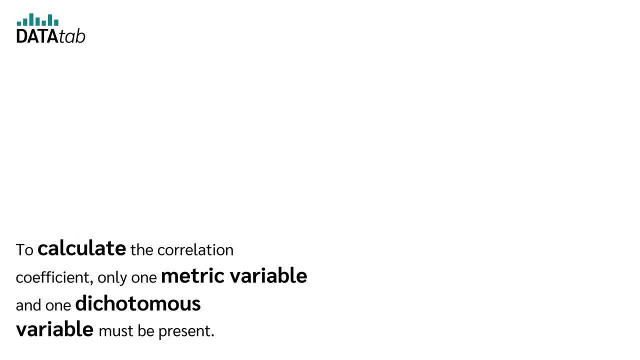 one metric variable and one dichotomous variable must be present. However, if we want to test whether the correlation coefficient is significantly different from 0, the one metric variable must also be normally distributed. If this is not, given the calculated test statistic. 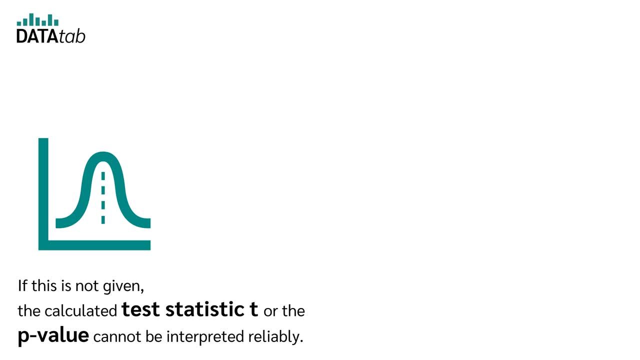 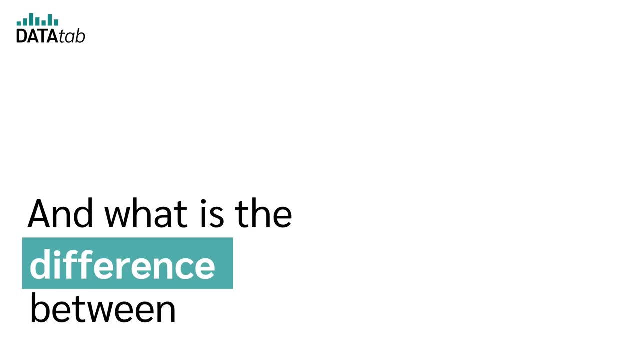 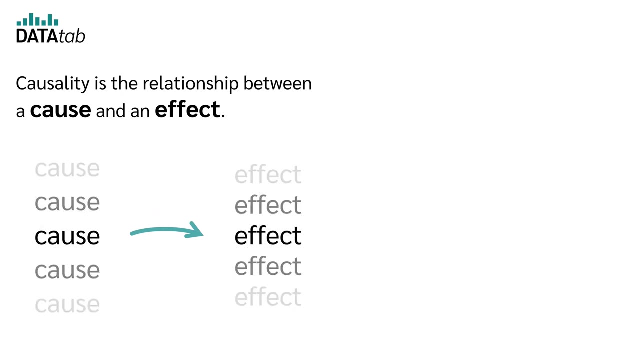 t or the p-value cannot be calculated. This brings us to the last question: What is causality And what is the difference between causality and correlation? Causality is the relationship between a cause and an effect. In a causal relationship, we have a cause and a resultant effect. 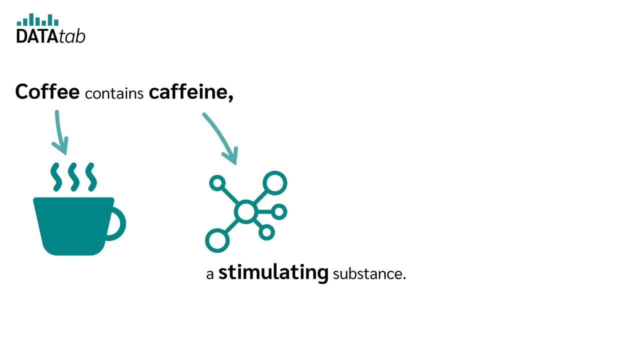 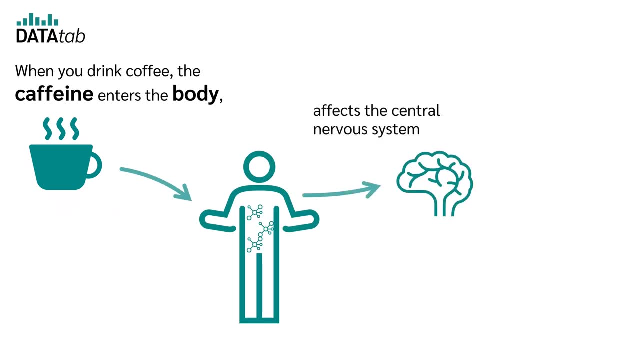 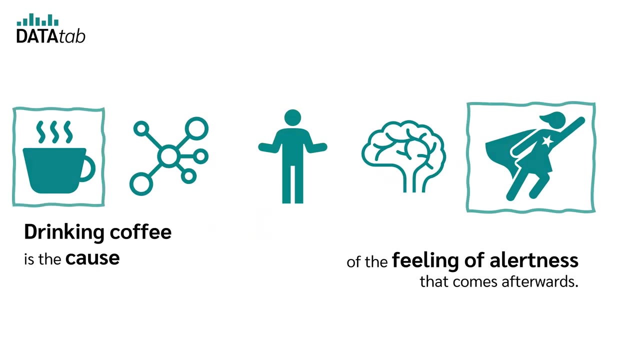 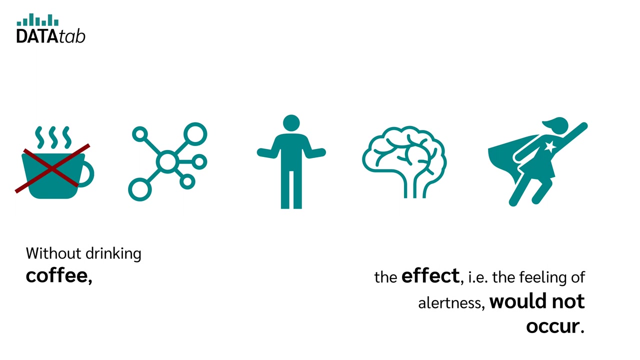 An example: Coffee contains caffeine, a stimulating substance. When you drink coffee, the caffeine enters the body, affects the central nervous system and leads to increased alertedness. Drinking coffee is the cause of the feeling of alertedness that comes afterwards. Without drinking coffee, the effect, ie the feeling of alertedness, would not occur, But causality. 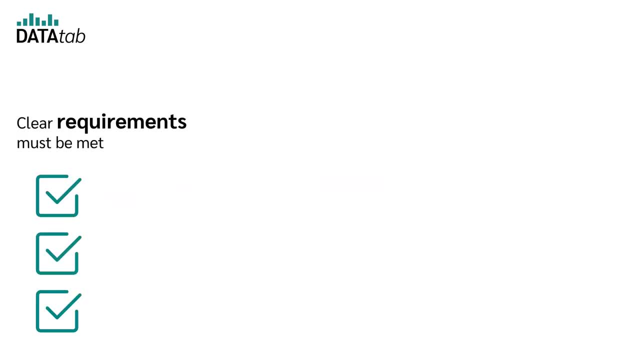 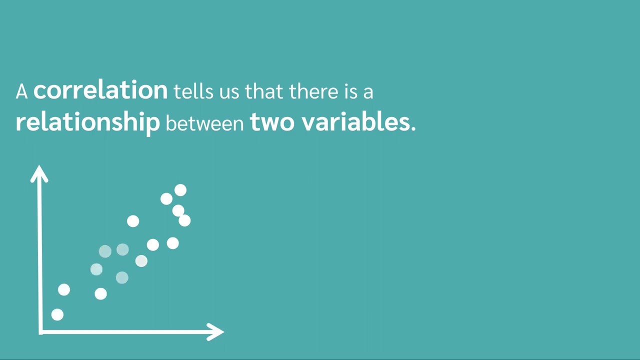 is not always so easy to determine. Clear requirements must be met in order to speak of a causal relationship, But more about that later. So what is the difference between correlation and causality? A correlation tells us that there is a relationship between two variables. 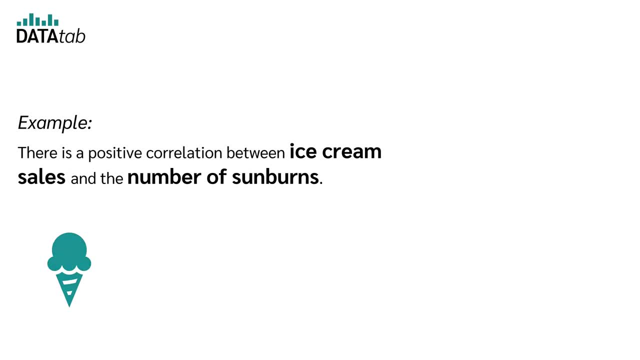 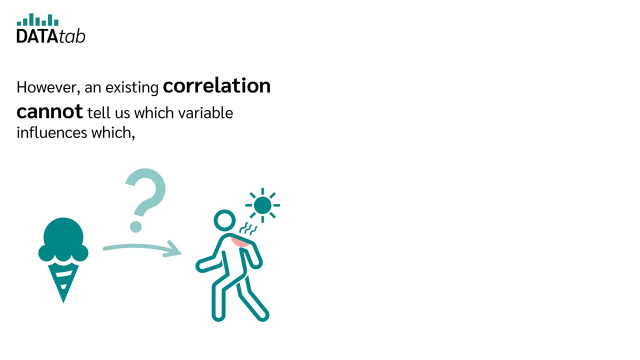 Example, There is a positive correlation between ice cream sales and the number of sunburns. However, an existing correlation cannot tell us which variable influences which or whether a third variable is responsible for the correlation. In our example, both variables are influenced by a common cause, namely sunny weather. On sunny days, people buy more ice. 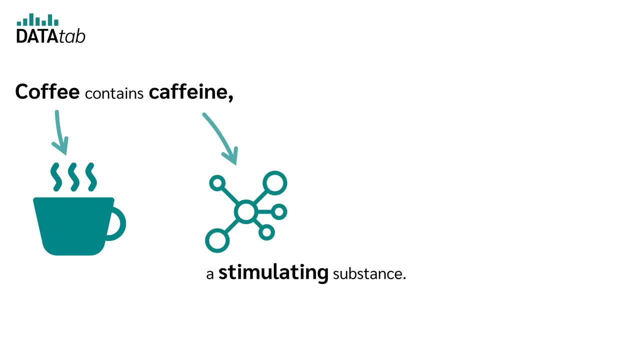 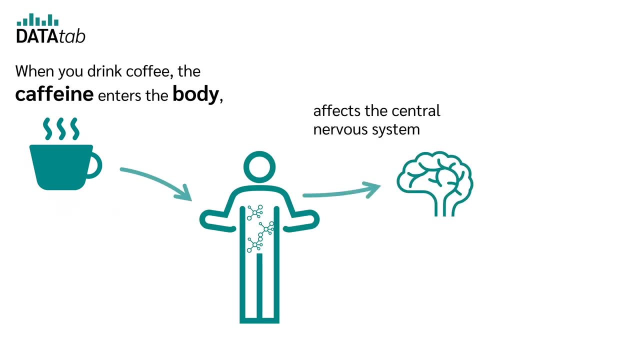 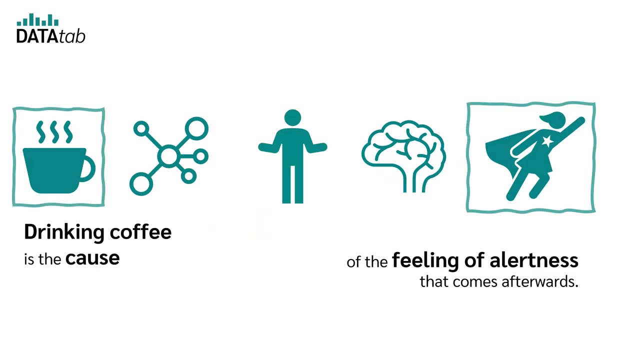 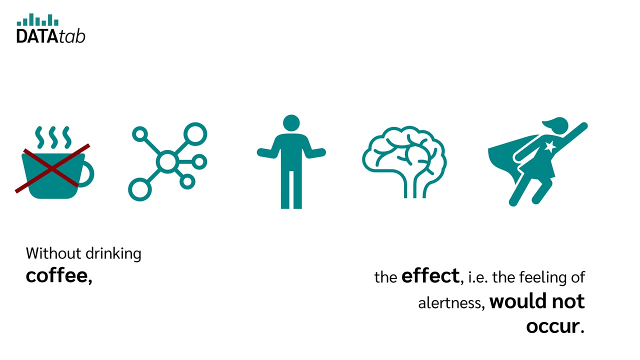 An example: Coffee contains caffeine, a stimulating substance. When you drink coffee, the caffeine enters the body, affects the central nervous system and leads to increased alertedness. Drinking coffee is the cause of the feeling of alertedness that comes afterwards. Without drinking coffee, the effect, ie the feeling of alertedness, would not occur. 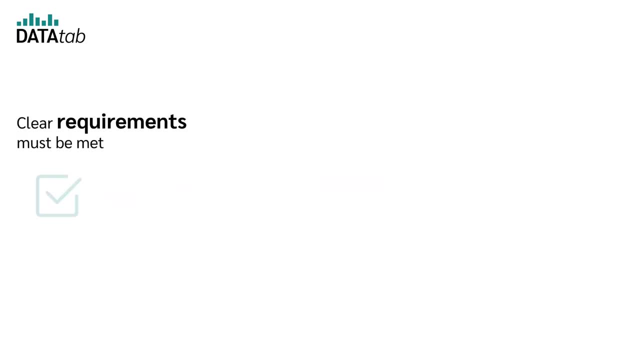 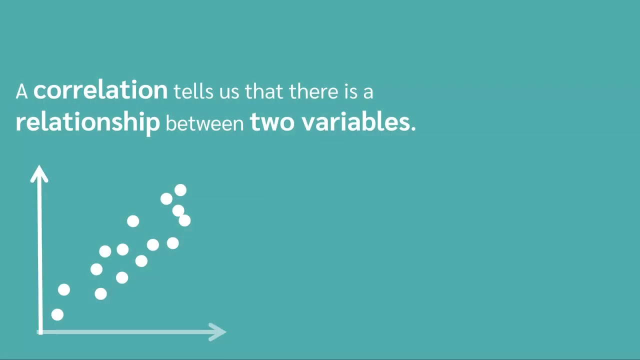 But causality is not always so easy to determine. Other requirements must be met in order to speak of a causal relationship, But more about that later. So what is the difference between correlation and causality? A correlation tells us that there is a relationship between two variables. 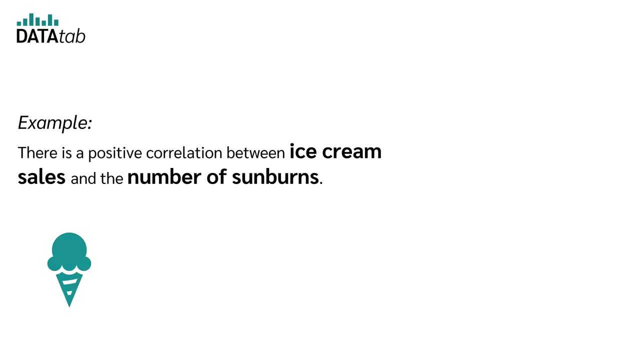 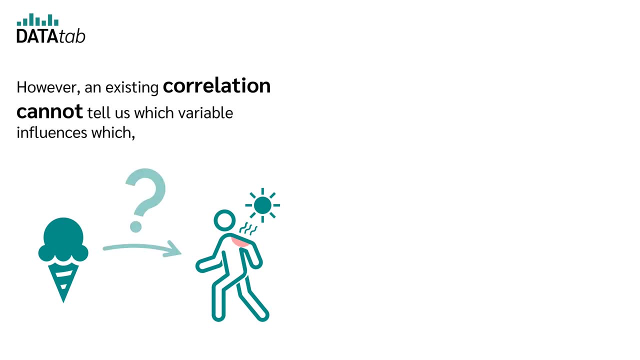 there is a positive correlation between ice cream sales and the number of sunburns. However, an existing correlation cannot tell us which variable influences which Or whether a third variable is responsible for the correlation. In our example, both variables are influenced by a common cause, namely sunny weather. 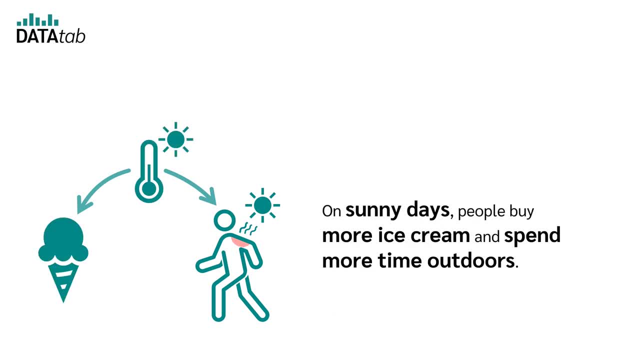 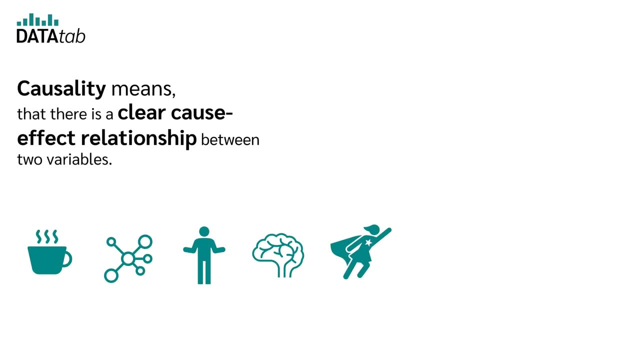 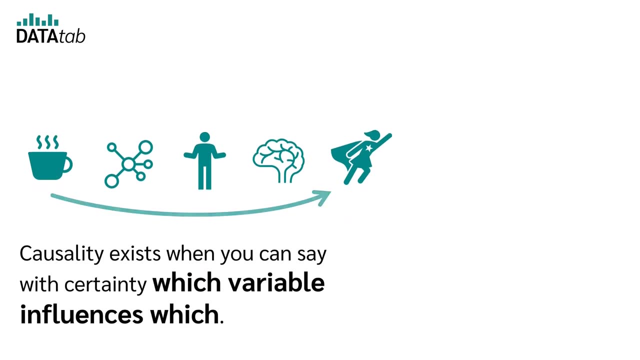 On sunny days, people buy more ice cream and spend more time outdoors. This can lead to an increased risk of sunburns. Causality means that there is a clear cause-effect relationship between two variables. Causality exists when you can say with certainty which variable influences which. 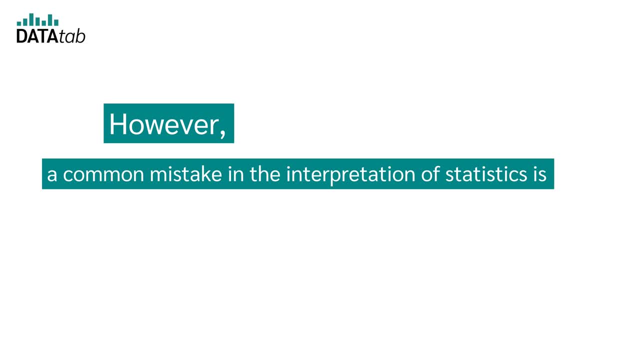 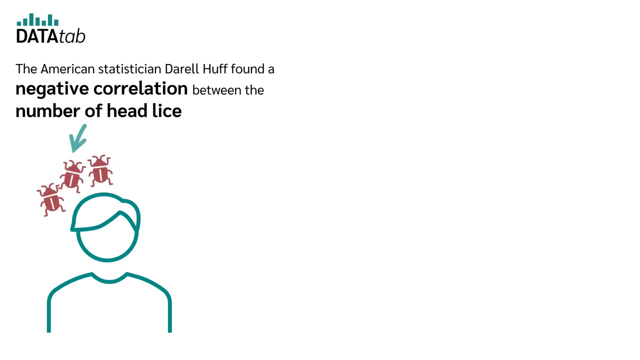 However, a common mistake in the interpretation of statistics is that a correlation is immediately assumed to be a causal relationship. Here is an example: The American statistician Daryl Huff found a negative correlation between the number of head lice and the body temperature of the inhabitants of an island. 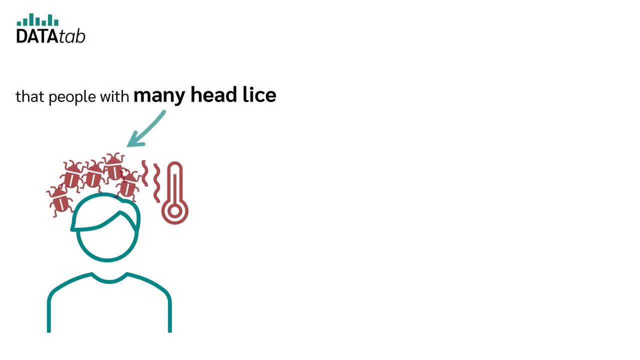 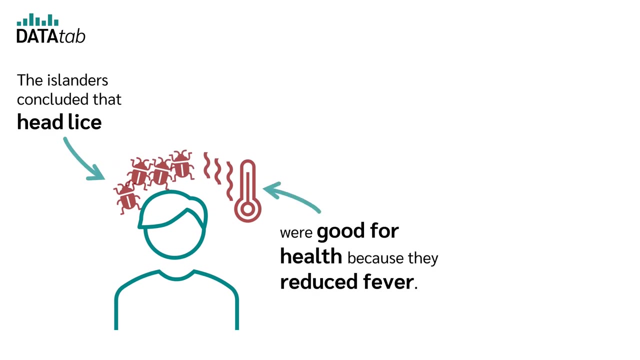 A negative correlation means That people with many head lice generally have a lower body temperature and people with few head lice generally have a higher body temperature. The islanders concluded that head lice were good for health because they reduced fever, So their assumption was that head lice have an effect on the temperature of the body. 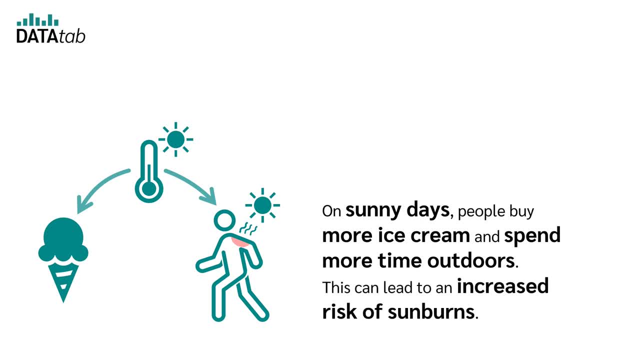 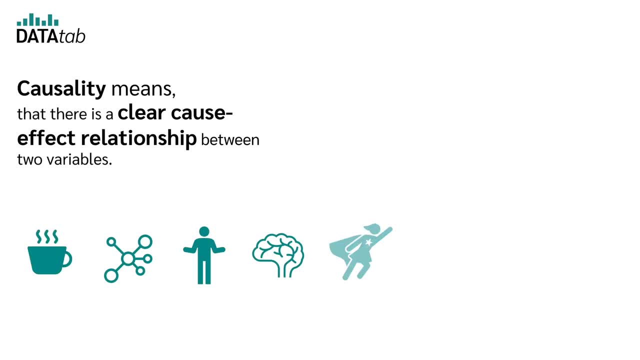 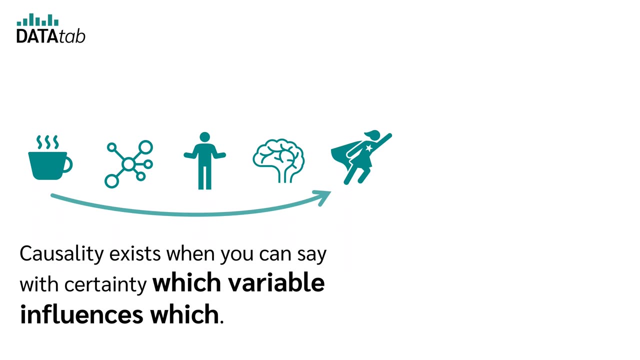 cream and spend more time outdoors. This can lead to an increased risk of sunburns. Causality means that there is a clear cause-effect relationship between two variables. Causality exists when you can say with certainty which variable influences which. However, a common 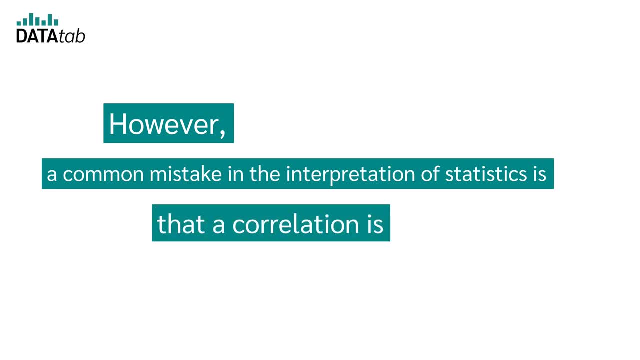 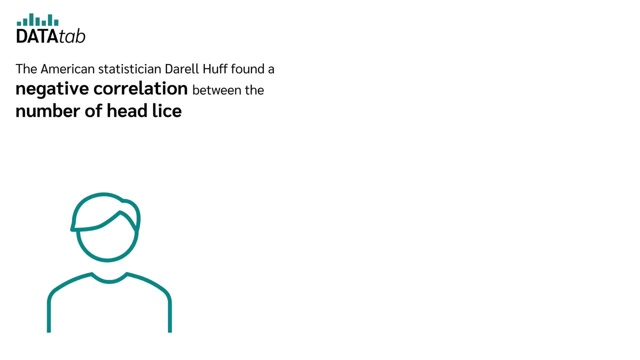 mistake in the interpretation of statistics is that a correlation is immediately assumed to be a causal relationship. Here is an example: The American statistician Daryl Hough found a negative correlation between the number of head lice and the body temperature of the inhabitants of an island- A negative 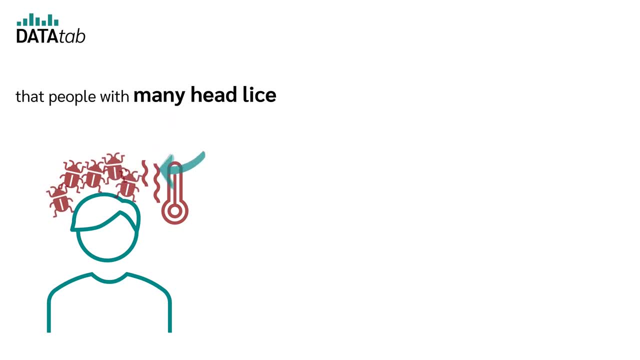 correlation means that people with many head lice generally have a lower body temperature and people with few head lice, less Head lice, generally have a higher body temperature. The islanders concluded that head lice were good for health because they reduced fever. 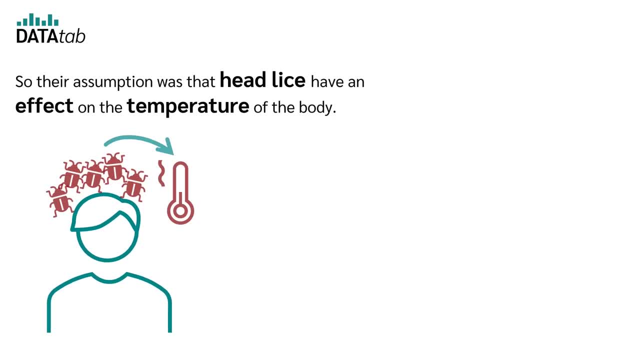 So their assumption was that head lice have an effect on the temperature of the body. In reality, the correct conclusion is the other way around. In an experiment it was possible to prove that high fever drives away the lice. So the high body temperature is the cause, not the effect. 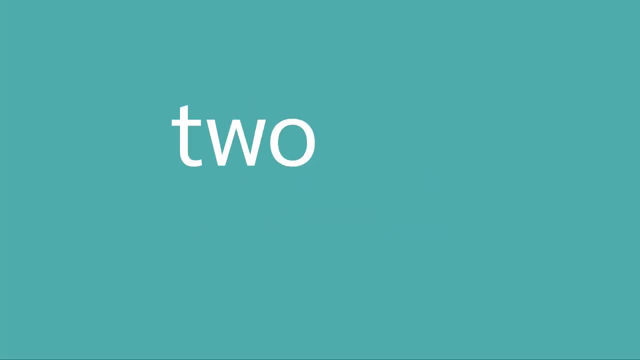 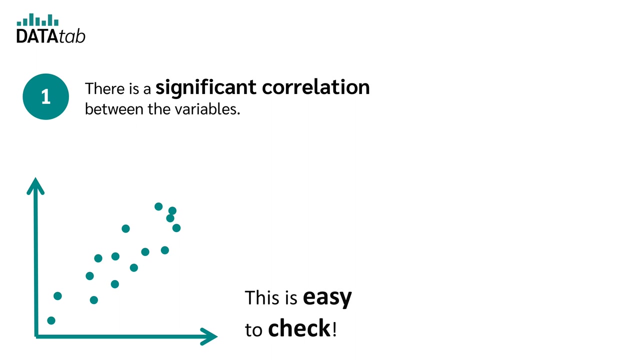 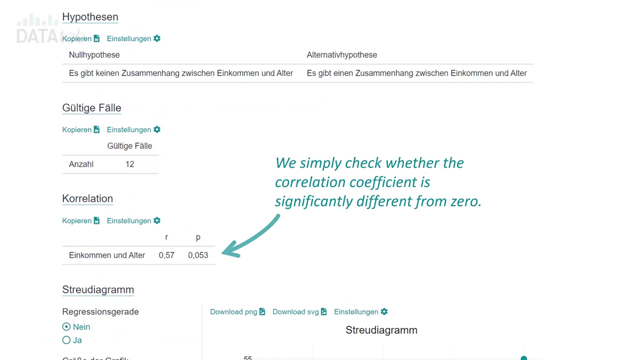 What are the conditions for talking about causality? There are two conditions for causality. Number one: there is a significant correlation between the variables. This is easy to check. We simply check whether the correlation coefficient is significantly different from zero. Number two: the second condition can be met in three ways. 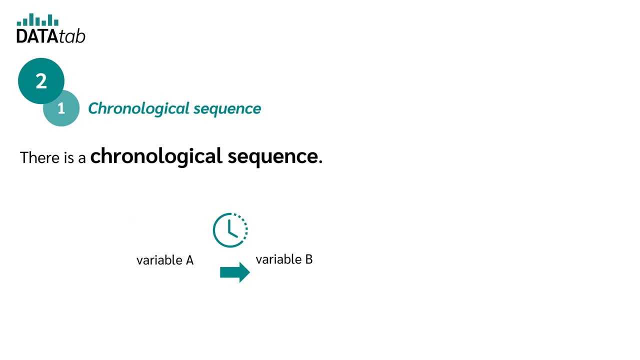 First, chronological sequence. There is a chronological sequence and the results of one variable occurred before the results of the other variable. Second experiment: A controlled experiment was conducted in which the two variables can be specifically influenced. And number three theory. There is a well-founded and plausible theory in which direction the causal relationship